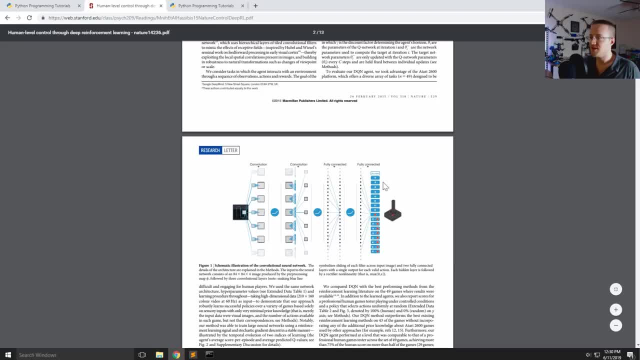 not this one- And then you've seen the following image. So this is how the deep query network, or deep Q network, is going to learn. So what's going to happen is: you've got this input- In this case it's an image- You've got some convolution layers- They don't have to be convolution layers. 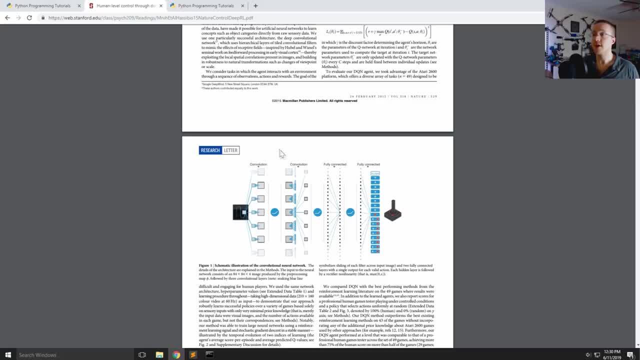 some fully connected layers. You don't have to have those, but you've got some sort of deep neural network. And then you've got your output layer, and your output layer is going to map directly to various actions that you could take, And it's going to do so with a linear output. 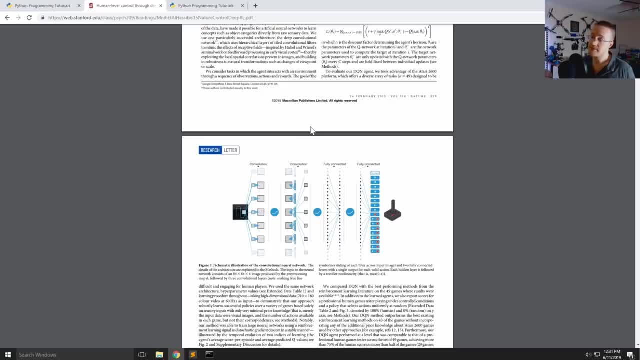 So it's a regression model with many outputs, not just one. Now, some people did try to do just one output per, so basically you'd have a model per possible action, but it doesn't really work well. And that's super, that's going to take a really long time to train, So anyways, here's another. 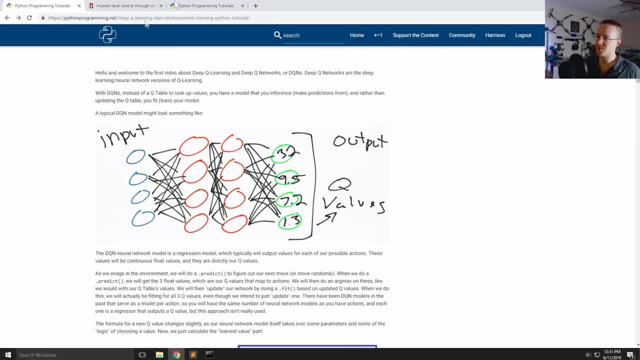 example. It's beautiful, really beautiful. You got input values, So again it doesn't have to be an image. You know this could be Delta X, Delta Y for the food, Delta X, Delta Y for the enemy, for example. 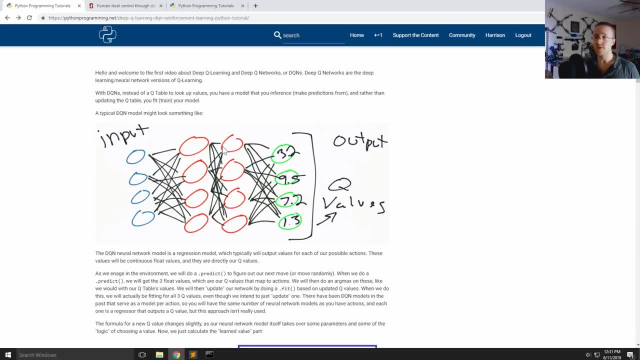 that could be your input. Boom, Then you've got your hidden layers Again. they could be convolution, They could be dense, They could be recurrent, whatever you want there. And then here you've got your output, again with a linear activation, So it's just going to output these. 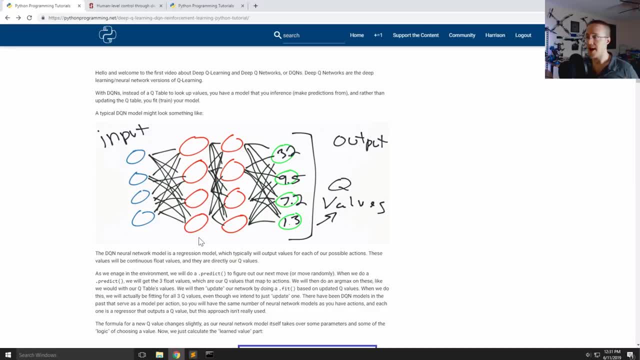 scalar values. Well, these are your Q values. They map directly to the various actions you could take. So in this case, let's say this was your output, You would take the argmax. Well, the argmax, or the max value, here is. 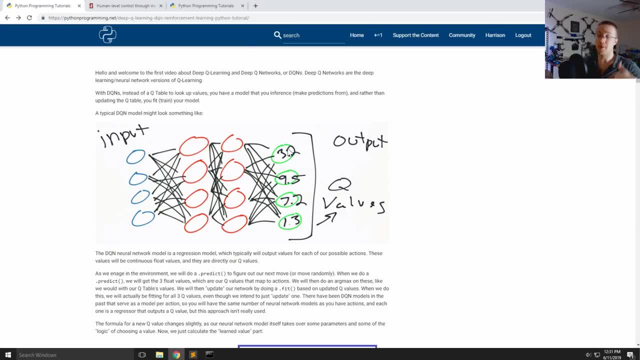 9.5 and the values are. you know, you're basically, if we were to map this and get the index values, it would be 0, 1,, 2, 3.. So argmax would be 1.. So whatever action 1 is, that would be the move that. 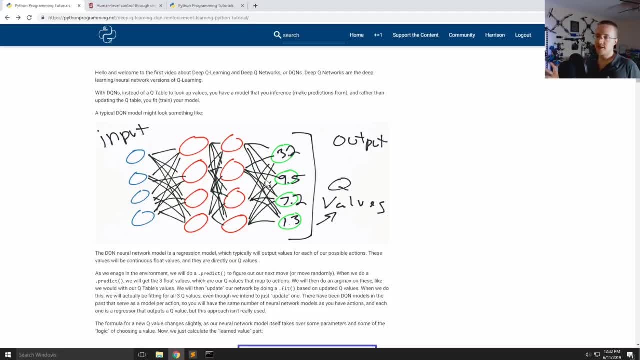 we would make Okay. So we've replaced this Q table with a deep neural network. The benefit here is we can learn way more complex Um environments. First of all, we can learn more complex environments just because a deep neural network is capable of actually mapping that also, a deep neural network can take actions. that it's. 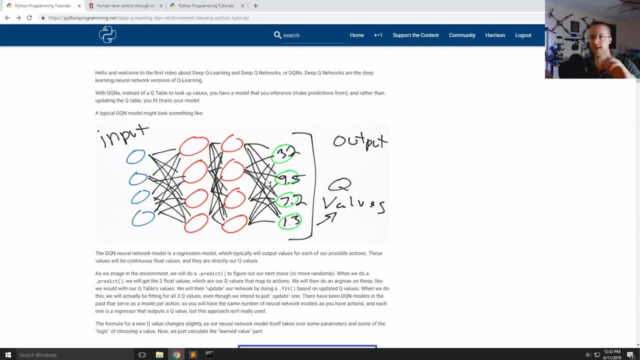 never seen before. So, with Q learning, if, a if, if a certain scenario presented itself and it was outside of any of the discrete combinations that we've ever seen, well, it's going to take a random action, because it got initialized randomly. A deep neural network, on the other hand, is not. 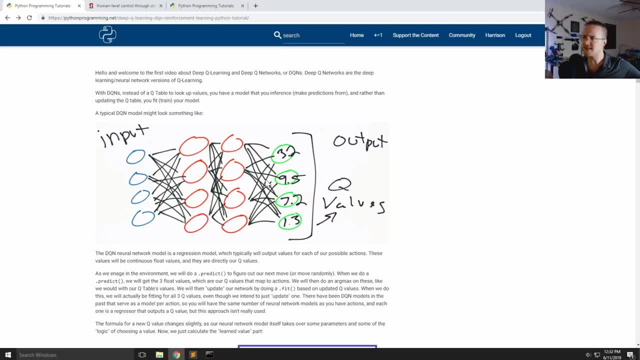 it can actually recognize things that are similar, but it's never seen this thing before and it can act accordingly. So, first of all, a deep neural network is going to do better in that case. So in that way it can solve for way more complex. 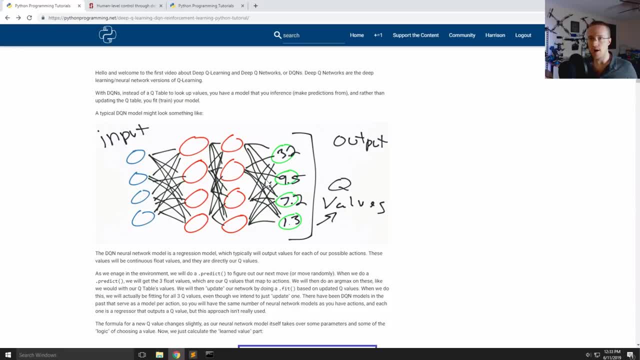 environments, but also, as we saw, as you just even barely increase that, that discrete size of your Q table, the amount of memory that's required to maintain that Q table, just just explodes right And it it, it both in in terms of your 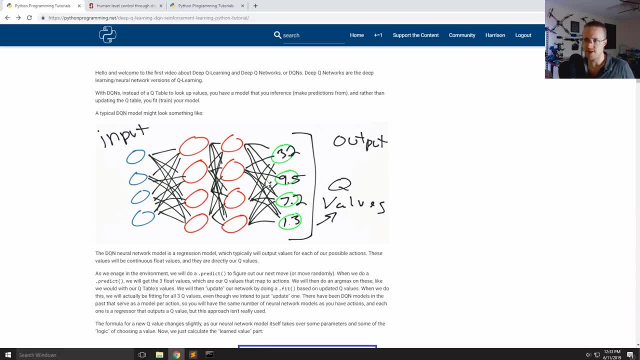 both your observation space size or your discrete observations based size, but also in your actions. So in our case, up to this point, we've only taken four. I'd like to introduce a few more actions moving forward, You know. so what we're going to do is we're going to keep the diagonal moves. 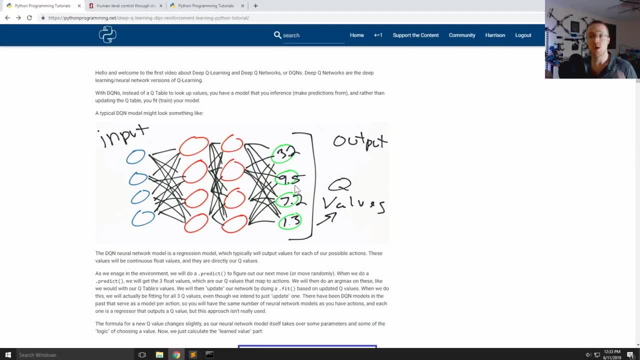 but also allow for just straight cardinal, like up down, left, right as well as don't move. So so we're going to introduce all of those as well, Anyway. so so for those two reasons, better the. the downside is neural networks are kind of finicky, so we've got to, we're going to. 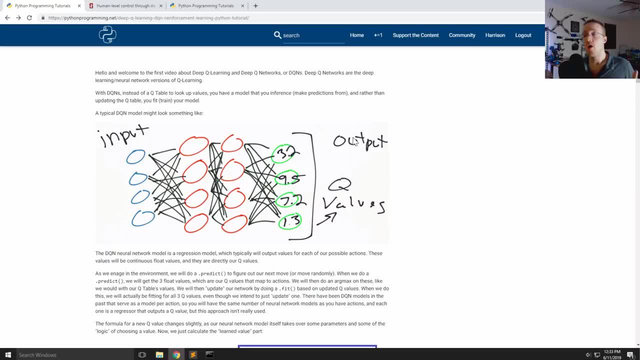 have to handle for a lot of things that are finicky about neural networks. also, it's going to take a lot longer to train. so on an identical model um or an identical environment, like in the blob env um where it took our q table minutes to to fully populate. basically it's just a brute. 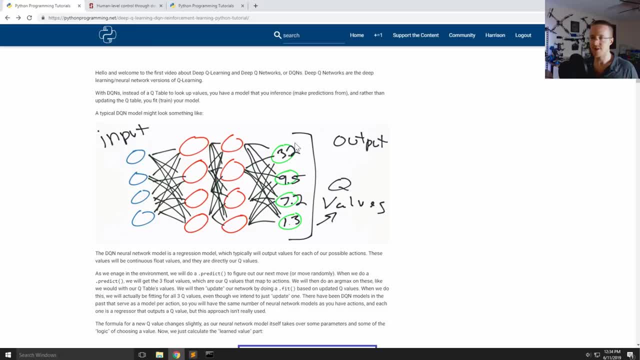 force operation basically. so if it's small enough, you know your cpu can handle it. um where it took. you know minutes for a q table. it's going to take hours for q learning um, but the benefit is where it takes. i'm sorry it's going to take hours for deep q learning um, but the benefit here is for. 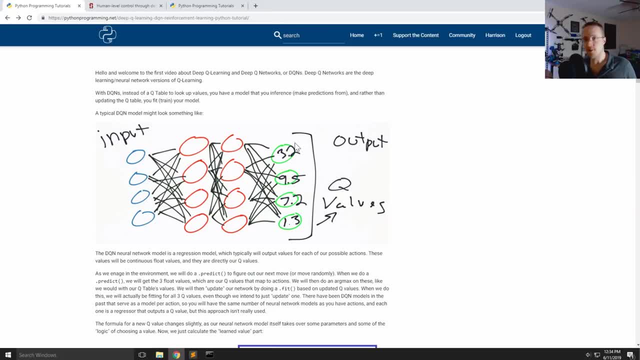 certain environments where it takes, yes, a long time, like weeks, for deep q learning to to learn an environment. uh, it would require, you know, petabytes of memory for a q table to figure it out. okay, so so that's that, there's your difference. so, really, they're going to solve different types of environments and, honestly, q learning is pretty. 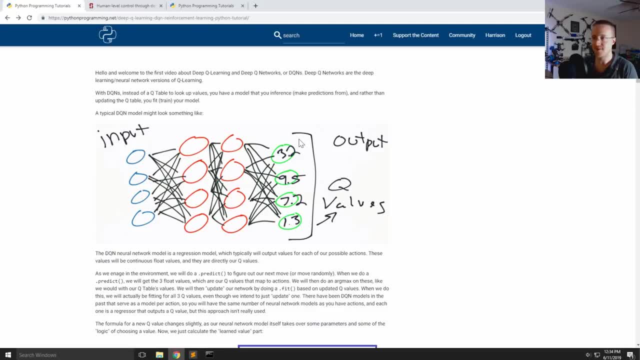 much useless. you can use it for cool novel, little niche things, for sure, uh, but you're not going to find too much use for it in the real world, i don't think, whereas deep q learning, you can actually start to apply it to really cool things. so, anyways, enough jibber jabber. uh, the last concept i want. 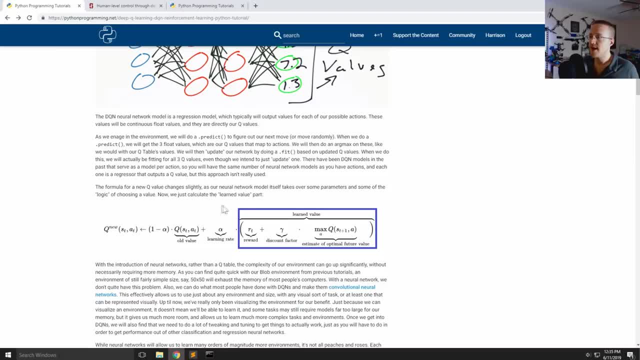 to do before we get into. uh, actually writing code is right here. this learned value change. so before we get into this whole thing, whereas the neural network kind of solves for this, like learning rate and all that and and just updating values, this is solved through back propagation and fancy. 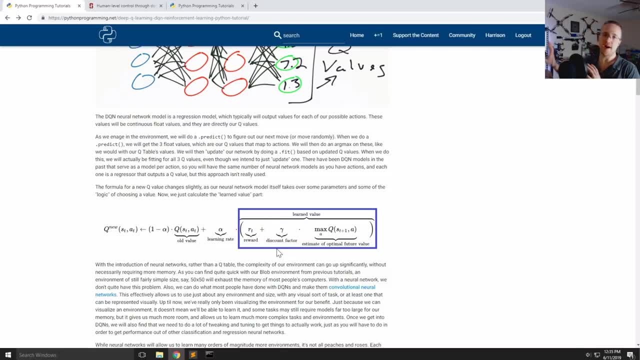 things, but we still want to retain the future values, because neural networks don't care. they don't give a heck about future. they care about right now. what is this thing, what is this exact value they don't care about? well, what does this chain of events do other than a recurrent neural 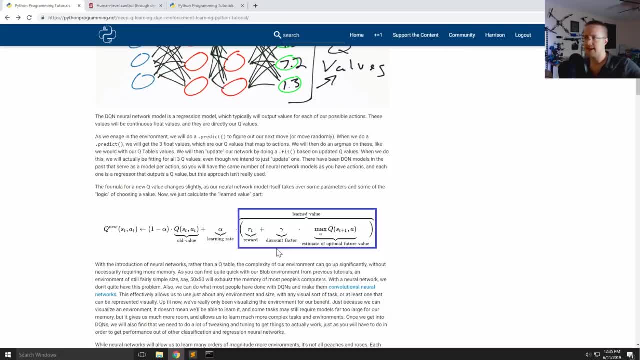 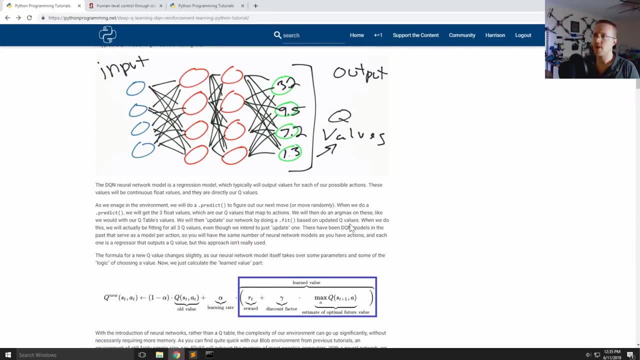 network, i suppose. but really, a recurrent neural network cares about the history, not the future. so, anyways, in this case, uh, we still want to retain this, so we are still going to use this and basically the way we're going to do this is: every step this agent takes, we still need to. 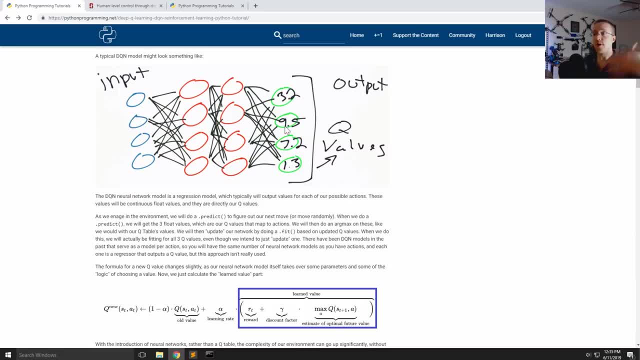 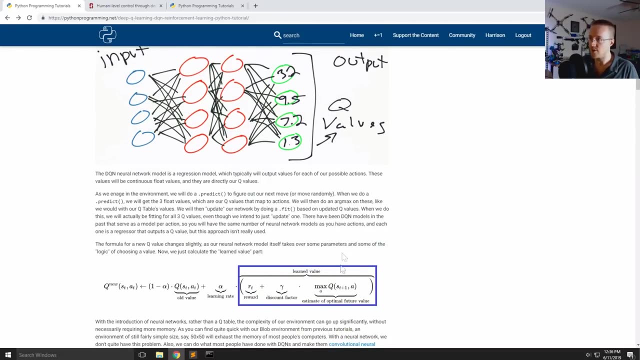 update that q value. so what we're going to do is we query for the q value, we take that action or a random one, depending on Epsilon, then we- you know, we re-sample the environment, figure out what our you know what the next reward would be here, and then we can calculate this new q value. 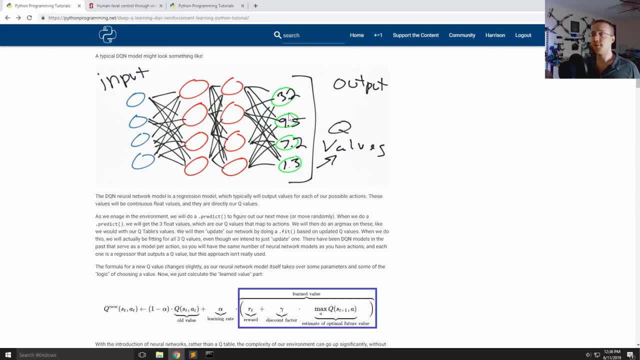 um, and then do a fit operation. so people who are familiar with deep neural networks are already like, wow, that's a lot of fits. yep, sure is also. that's one fit at a time. so, as you're going to see, when we go to write this code, we actually have to have to handle for that as well, because that would 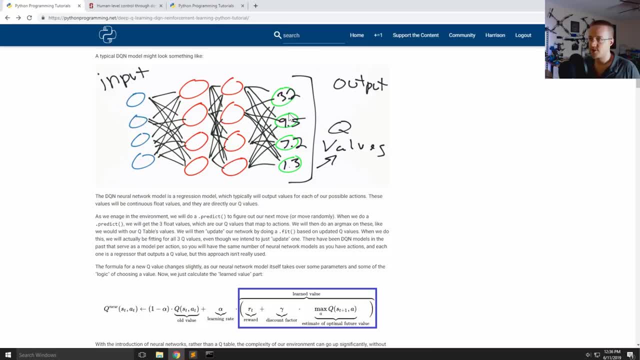 make for a very unstable neural network. um, so there's two ways that we're handling for that, but with that I think we're just going to jump in the code. um, because I think it'll make more sense. you just code, coding it and covering it as we get to those points. 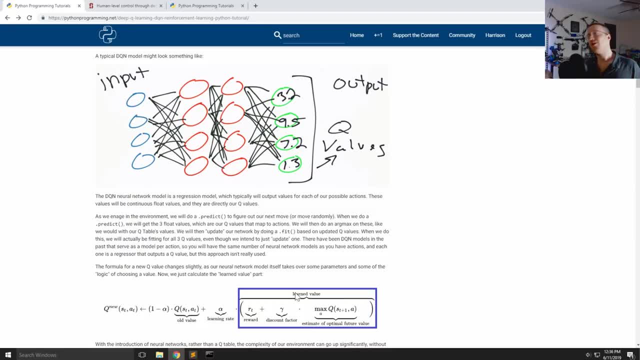 um, okay, so hopefully that was enough information. like I said, all the tutorials I've ever seen on deep Q learning um have been terrible and there's like so much information that's left out um that you know to get the overarching concept. honestly, this picture is enough. 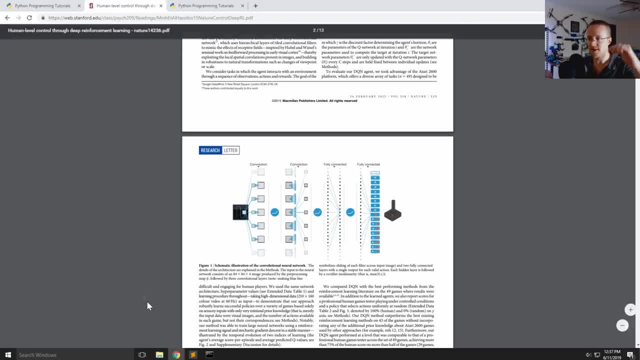 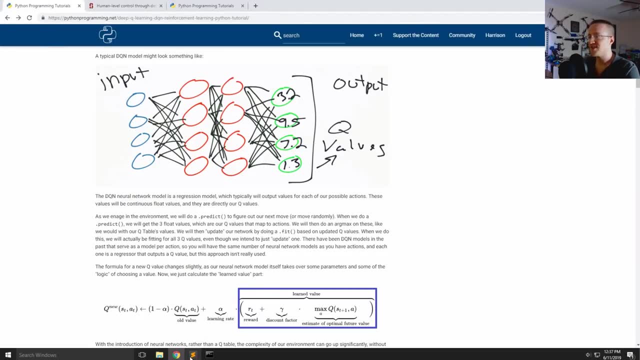 uh. but then when it comes time to actually look at code and how it really will work- like can you sit down and code it after you read someone's tutorial? my hope is you really can after this one, but otherwise I don't think a tutorial exists for doing it. 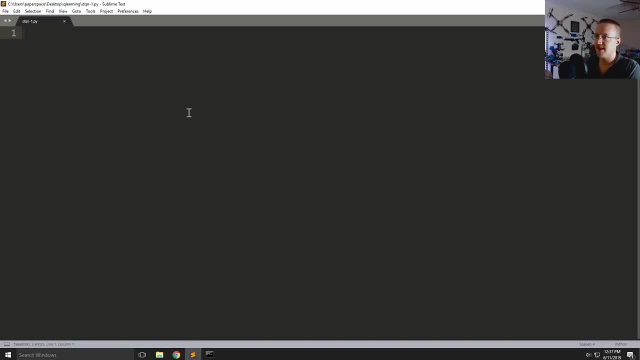 so. so anyways, uh, let's get started. so the first thing we're going to do is I'm going to uh create, we're going to at least hopefully code our agent, uh, at least the model and talk about some of the parameters, and then, probably in the next tutorial, we'll do fitment and or training, basically, and 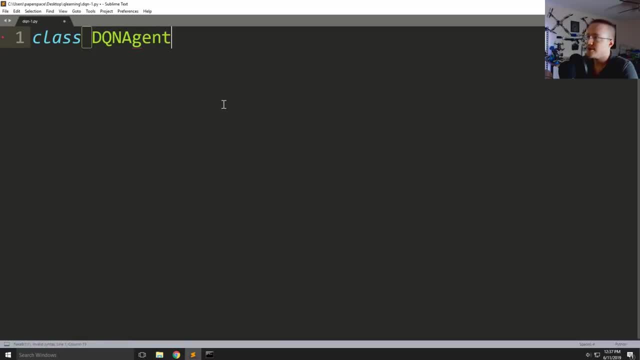 all that. so, anyway, class dqn agents and this agent: uh, let's just do define, create model first. this should be fairly basic, it's just going to be a convnet. we don't have to do a convnet, I'm just going to do one, just so you can more easily translate this. 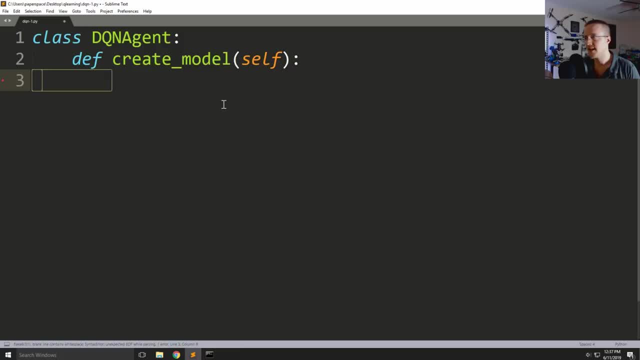 to something else. so the first thing you should do anytime you learn something, is: go try to apply it to something else. so try it, and then you'll meet it, because you it might make sense to you, as you're listening to me talk about it, but then you go to try to apply it and then suddenly it. 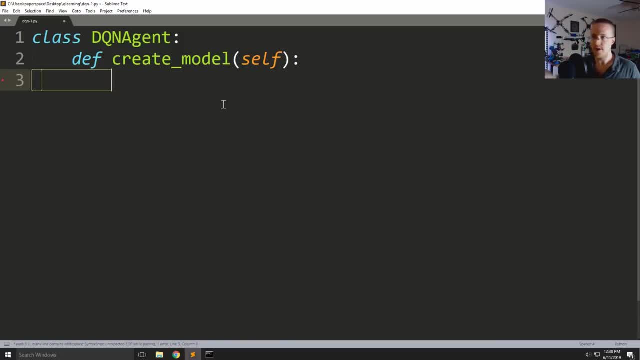 doesn't work, or you're confused, or you realize: oh, I don't really actually know how to do this. so, anyway, the first thing you should do, try to apply it. someone complained recently about my drinking on camera, uh saying they don't want to hear me gulp. 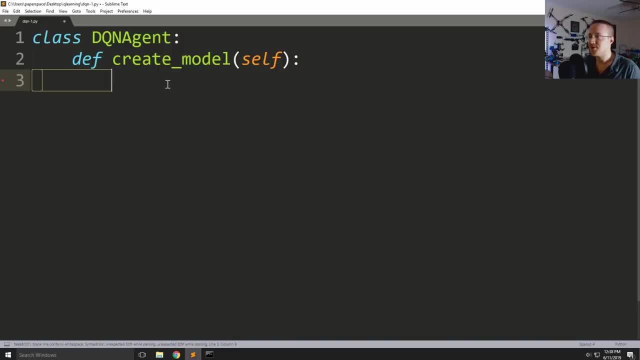 um, I'm drinking because my mouth is dry and the most annoying thing ever is listening to someone talk with a dry mouth. so, uh, you're welcome, jerk. so anyway, um, create model, okay. so, uh, we'll start with. model equals a sequential model, and now let's go ahead and make some imports. so, uh, the first. 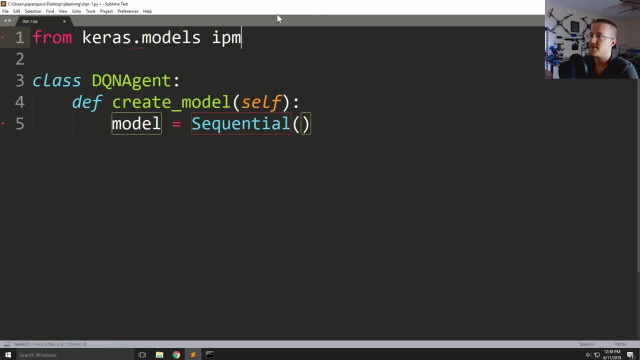 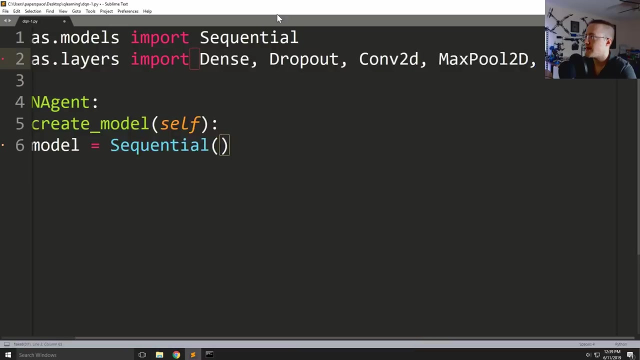 thing I need to bring in is: from kerosmodels let's import, import sequential. and uh, then we're going to say: from keroslayers let's import dense dropout conv 2d max pool, 2d um activation, activation flatten. I think that's everything. sorry, that ran over my face. 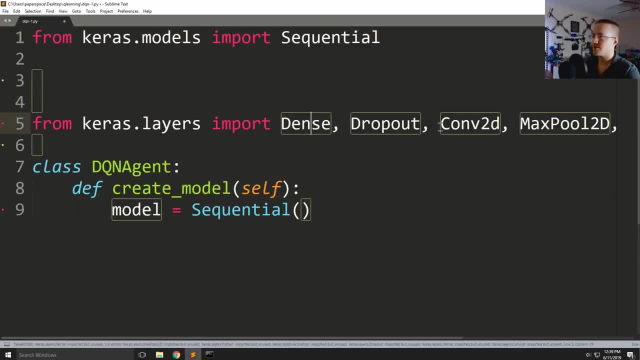 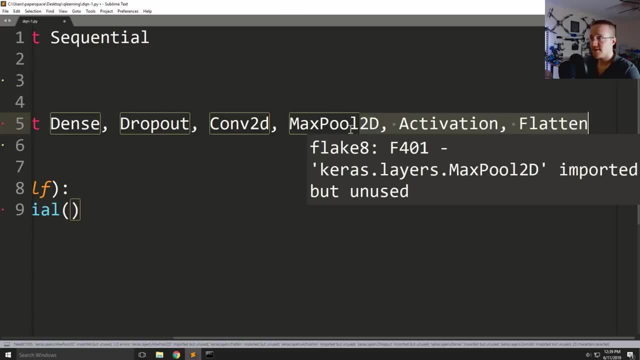 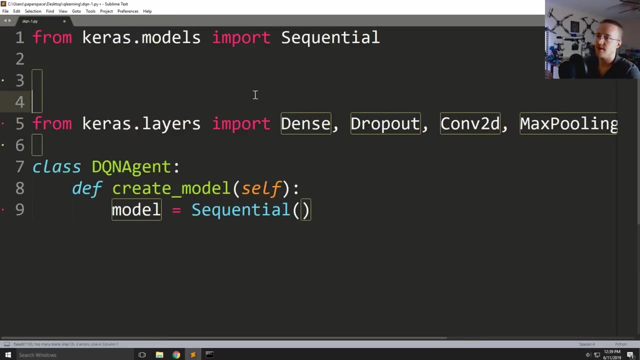 my bad. anyway, there we go: dense dropout conv duty duty, max pool 2d, and actually that's max pooling 2d. activation and flatten. okay, those are all of the imports. also the. you can always go to the text-based version of tutorials if code runs over. 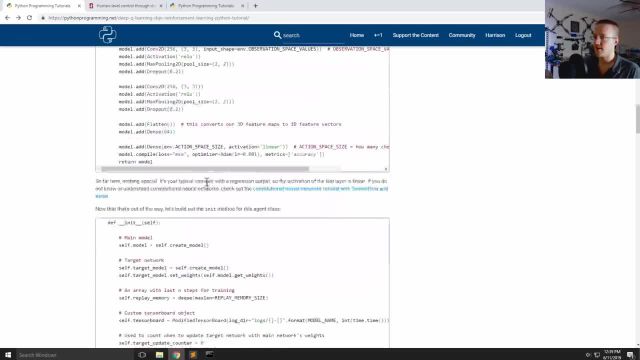 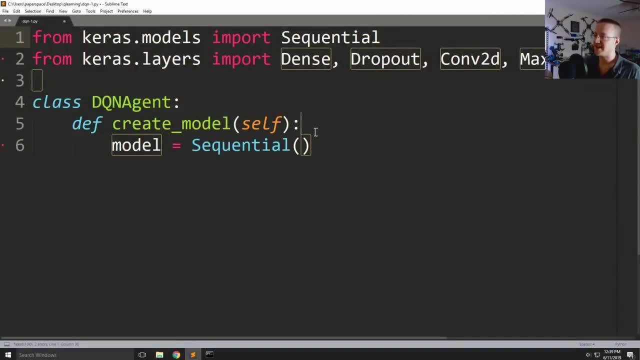 my ugly mug. um, you can check those out. actually, I don't even know, maybe at the very end it'll be there anyway, by the time I made it it'll be there anyways. um, okay, so we got that stuff. um, the other thing, I'll go ahead. 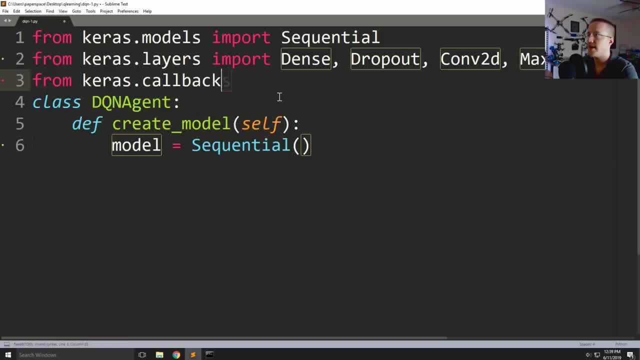 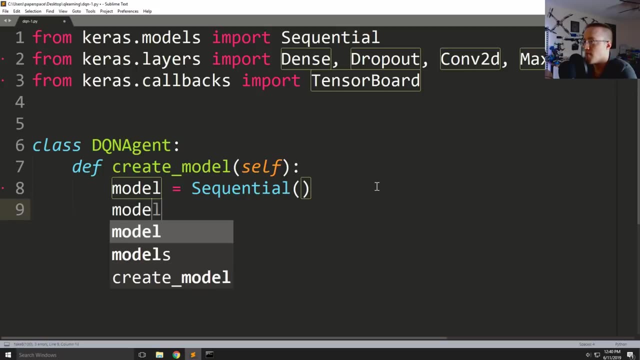 and import to is from keroscallbacks, let's import tensor board. um, we need other things, but I want to cover them when we get there. so model is equal to a sequential model. then we're going to say modeladd and then we're going to start adding a con. 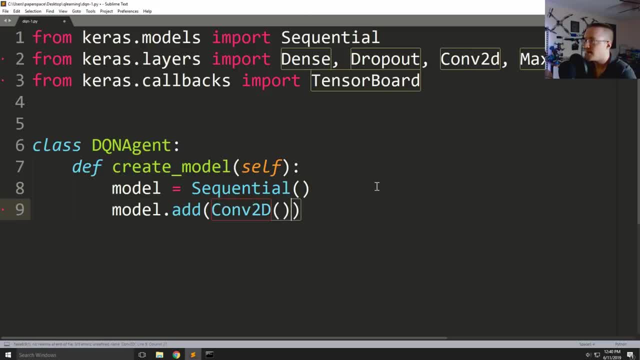 2, capital D. Let me fix that as well. Cool Conv 2D, which will give us 256 convolutions and the convolution window will be a three by three and then input underscore shape And this is going to be equal to. it will say envobservation space values. 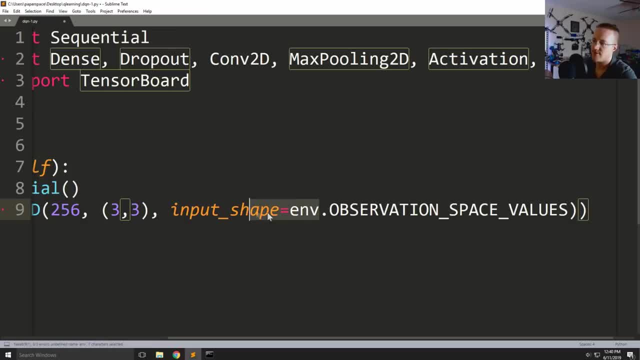 And then close this off And this doesn't quite yet exist. We have to create the environment. I'm still a little uncertain if I'm going to actually rewrite the environment, because it's converted to object oriented programming. now I may not actually like. we might just copy and 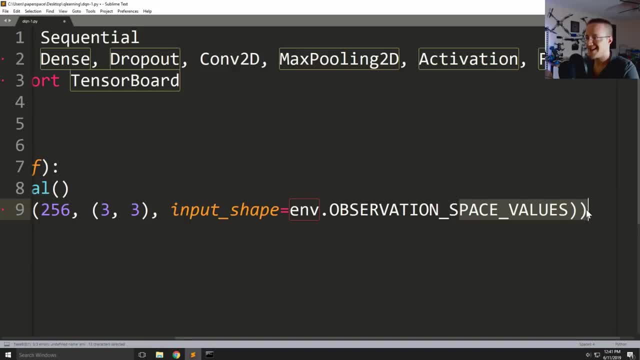 paste the updated environment. I'm going to copy and paste the updated environment And I'll just talk about it, because otherwise it'll take like an hour to go over that. So anyways, but we will. this will exist at some point in the near future. 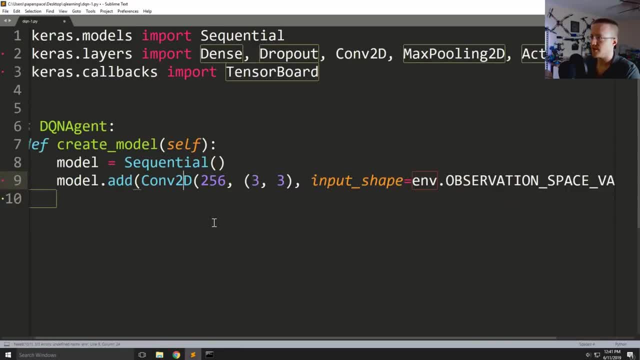 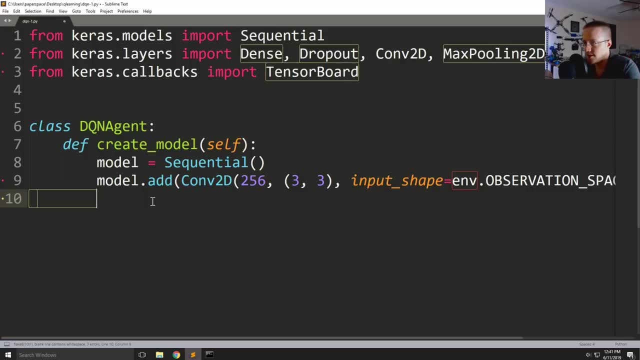 Then, once we've done that- I guess let me zoom out a little bit, since we're running out of space here- The next thing that we're going to do is we'll say modeladd, So that's our conv layer- We're going to add an activation, and the activation here: 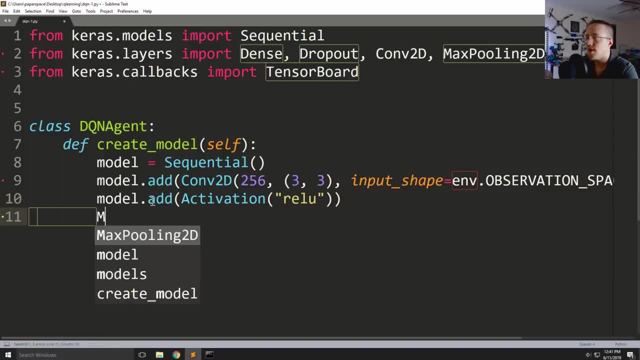 we'll use rectified linear And then modeladd max pooling 2D. We'll use a two by two window And, again, if you don't know what max pooling is, or convolutions, check out that basics tutorial because I cover it And I also have beautifully drawn photos If you really like my other photo. 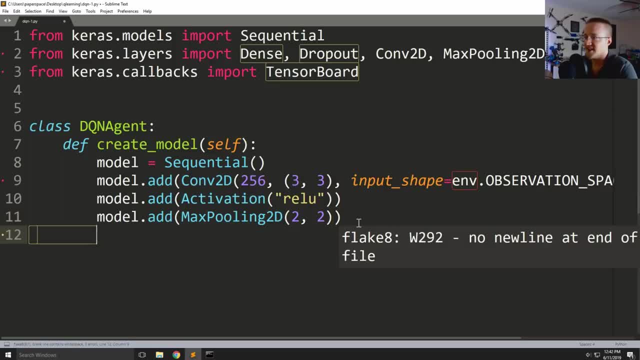 you'll love that, those photos. Then, after the max pooling, we're going to say modeladd, And we're going to add a dropout, And we'll drop out 20%, And then we're just going to do the same thing again. So this will: 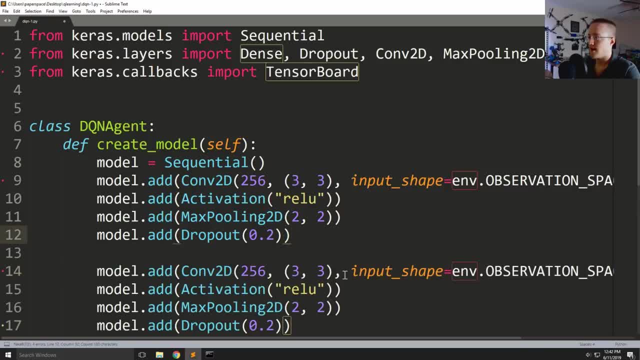 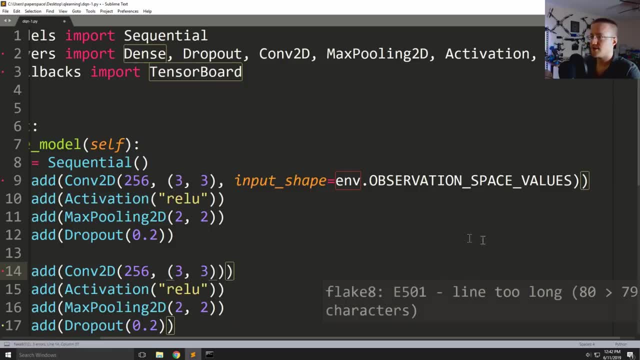 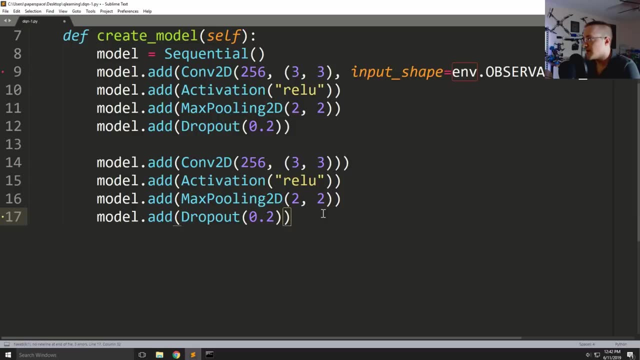 be two by two, 56. So copy pasta. We don't need to include the environment shape or the input shape, rather. So I'll do this. So two by two, 56, then we're going to say modeladd, We're going to 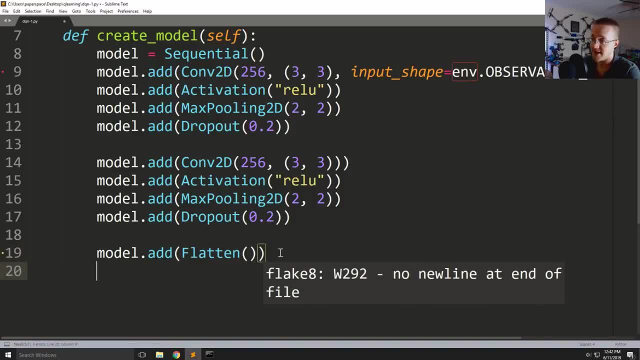 do a flatten here so we can pass it through a dense layer, And then we're going to say modeladd, And then we'll say modeladd, We'll throw in a dense 64 layer And then finally modeladd, a dense layer, And it'll be envaction space size And then the activation will be linear. 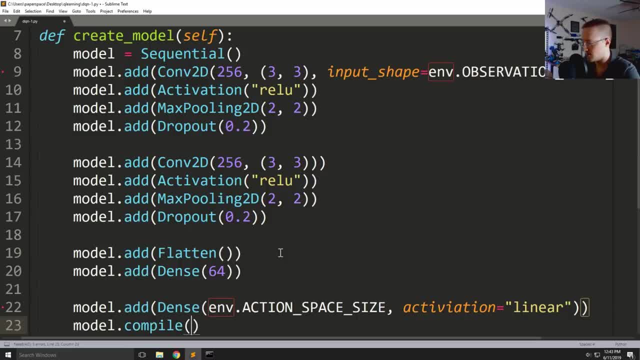 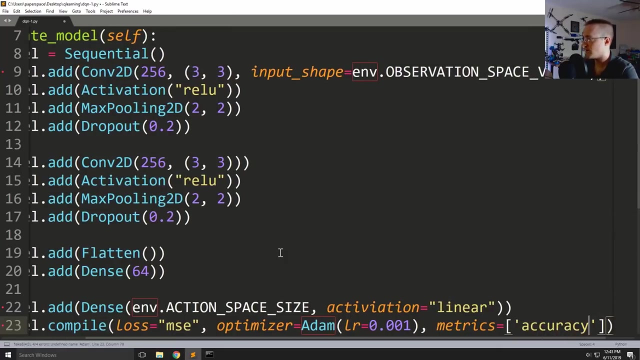 And then modelcompile And we'll say: loss is MSE for mean squared error. Optimizer will be the atom optimizer with a learning rate of 0.001.. And then metrics: we will track accuracy. Okay, So that is our model. 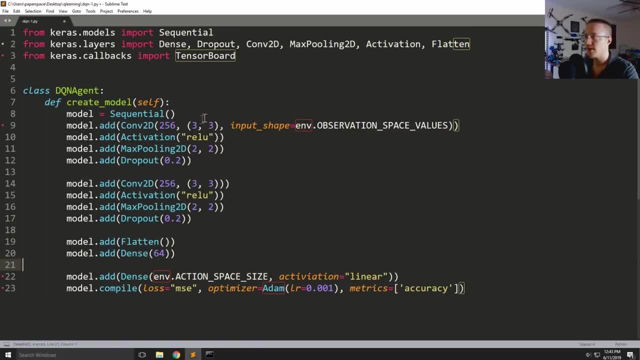 Again, sample code is in there. There'll be a link in the description to the sample code, So if you've missed anything, you can check that out. Okay, So, and then atom. we don't actually have atom imported, So let's go. 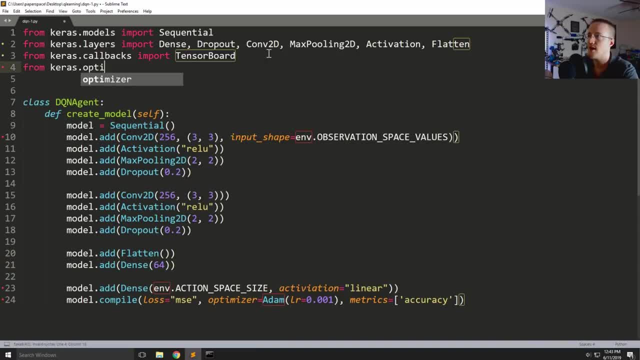 ahead and grab that as well. So from karosoptimizers import atom. Just for the record too, if anybody's watching this in the future, this is still TensorFlow like 1.15.. I don't know. Speaker 1.. Speaker: 2. Speaker, 3. Speaker, 4. Speaker, 5. Speaker, 6. Speaker, 7. Speaker, 8. Speaker, 9. Speaker, 9. Speaker, 10. Speaker, 11. Speaker, 12. Speaker, 11.. 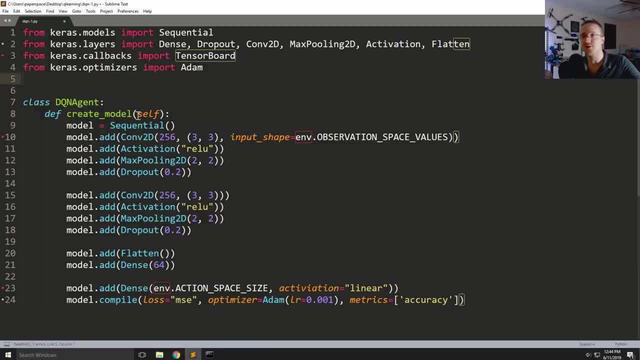 Speaker 12. Speaker- 3. Speaker 12. really know, actually i don't know what version i'm on, but it's not tensorflow 2 yet, uh, so keep that in mind. so some things might change by then. uh, and if it has changed, check the comments um. 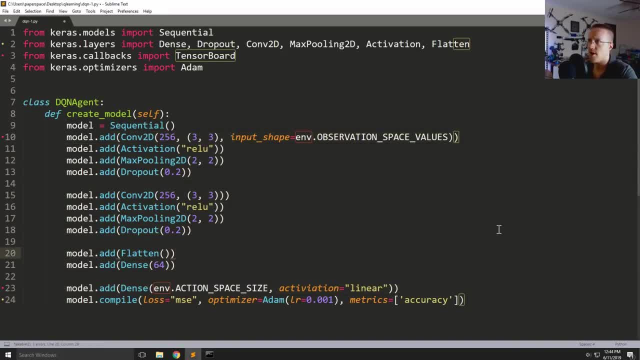 and then when it finally actually does truly matter what version of tensorflow i'm on, i will let you guys know. it's also kind of expected that you guys will know how to install tensorflow and keros. i'm not going to cover that again, for that go to the basics tutorial. so anyway, 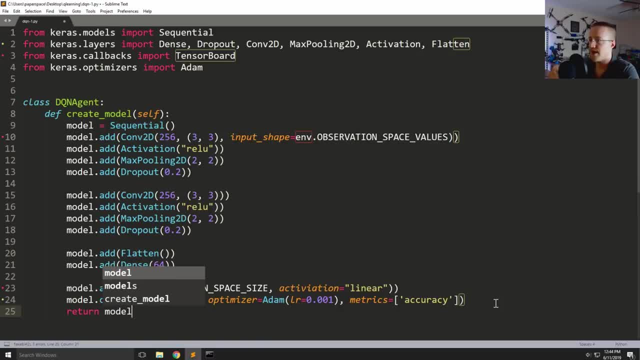 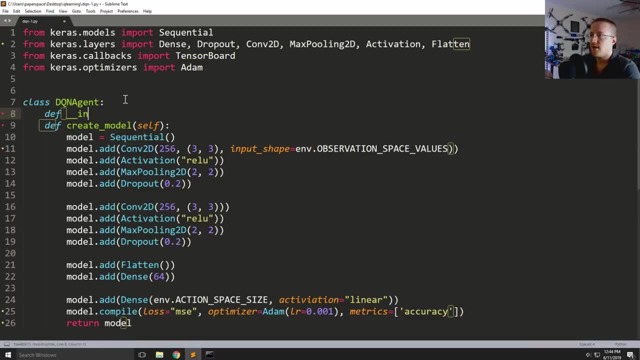 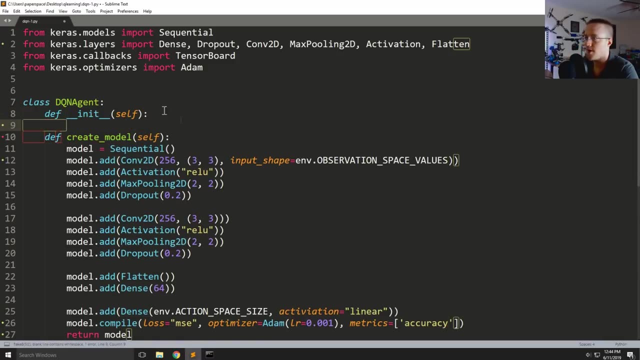 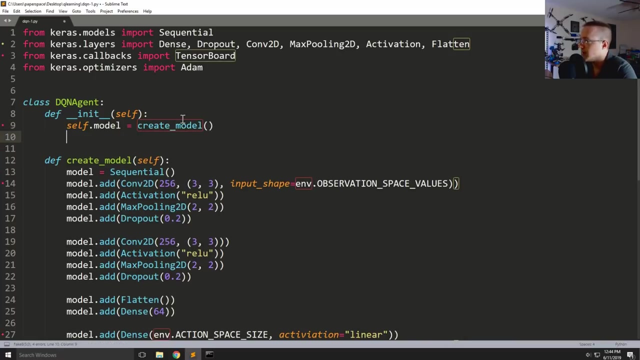 model compile. okay, then we will return that model. okay, so that's our model. then, uh, define in it self. and then now we're going to do the init method for this model. so we're going to say: self dot model equals, create underscore model. and then so that is going. what is your problem? 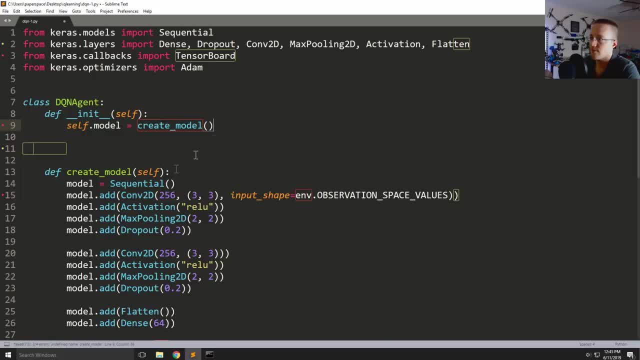 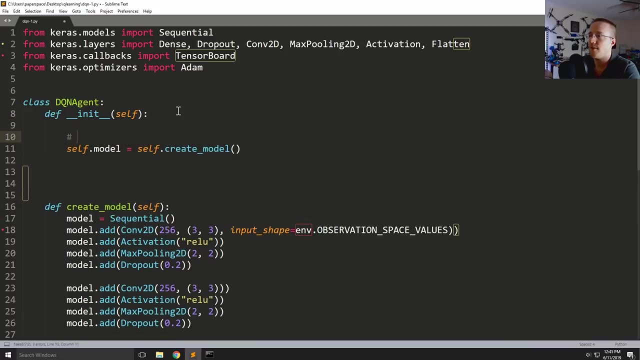 why are you unhappy? what? what the heck am i missing? oh, self dot- create more coffee is definitely necessary. okay, self dot model is create model, so that is that's going to be our main model. but then we need what's going to be called our target model. what the heck set dex? let's write that first. so self dot- uh, we'll call this target. 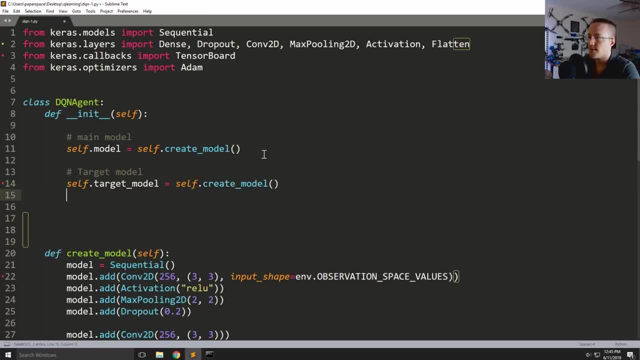 model equals self dot create model. but then we're going to say self dot target model dot set underscore weights and we want to set the weights to be exactly the same as selfmodelget underscore weights. okay, so what's going on here? so we we are going to wind up having two 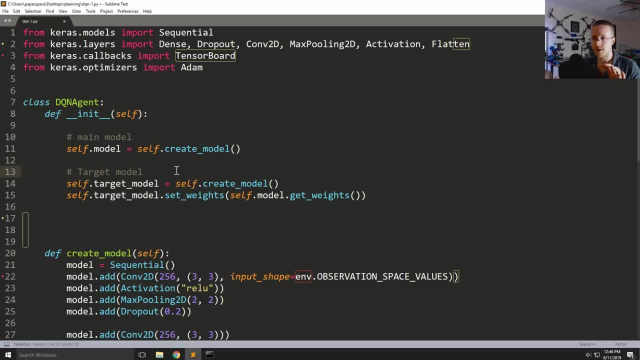 models here, and the reason why we want to do that is kind of there's. there's a few reasons, but mostly it's because this model is going to be going crazy. so first of all, we init the. the model itself is initialized randomly, as all neural networks are. 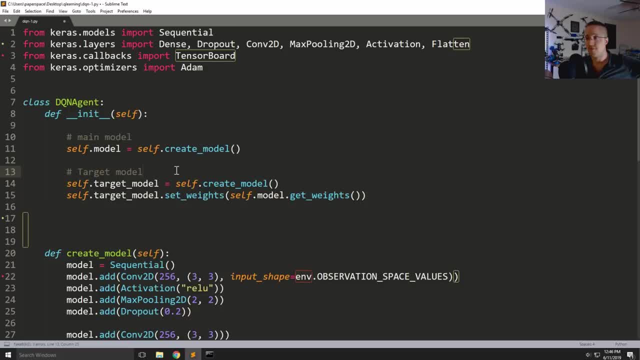 but we also are going to initialize with an epsilon, likely of one. so the um, the agent, is also going to be taking random actions, meaningless. so initially this model is going to be trying to fit to a whole bunch of random and that's going to be useless. and but eventually, as as it's, 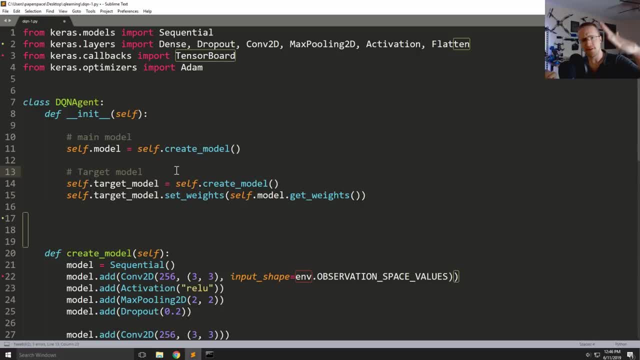 explored as it's gotten rewards, it's going to start to hopefully figure something out. but the problem is we're doing a dot predict for every single step this agent takes and what we want to have is some sort of consistency in those dot predicts that we're doing, because, besides doing a dot predict for every single step this agent takes and what we want to have is some sort of consistency in those dot predicts that we're doing, because, besides doing a dot predict, besides using dots Report shots of E, dubbed Um, that we're doing. bec excellent for us in the next part of this module. 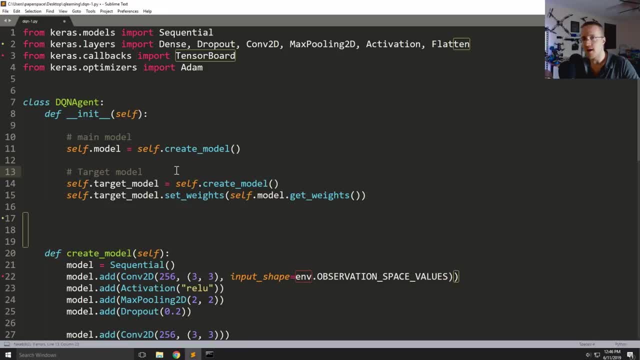 yeahTSWordFactoshut sketch 소개. Um, now I want any would be able to help us. putiation be already, i'm here. if someone actually gave you something for the next stage in the direction that I made you this half agеr, are you no moment givenzo? 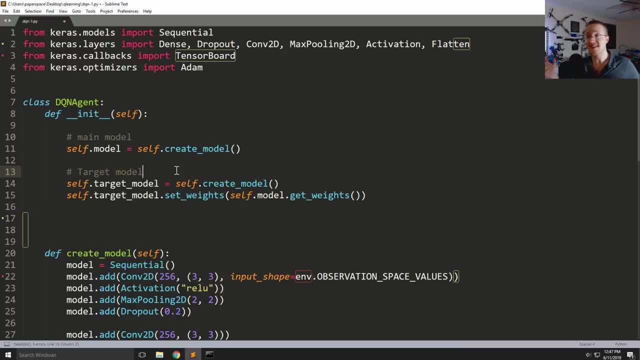 categories that we made it. doing a dot predict every single step. we're also doing a dot fit every single step. so this model, especially initially, is just going to be like all over the place as it's attempting to figure things out randomly. so the way we're going to compensate for that is we're going to have two models. so 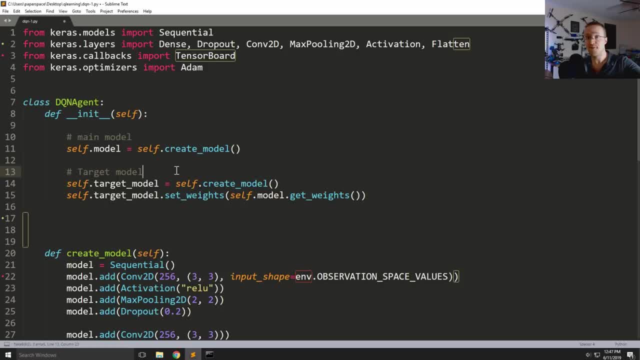 we've got self dot model. this is the model that we're dot fitting every step. and then we have self dot target model. this model we're this is the one that we're doing- a dot predict every step. and then i would even say: this is this is what we dot predict against every step. and then this is: 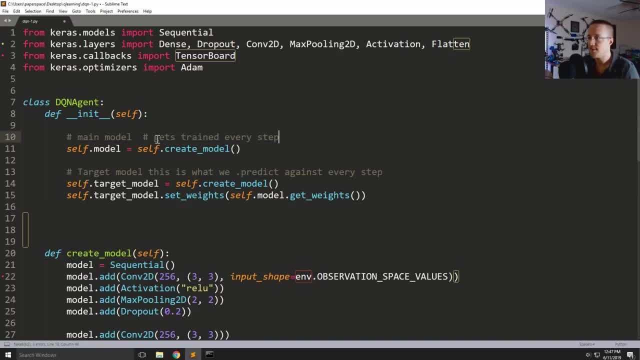 the one that gets you know, gets trained every step. make note of that because you'll probably forget so. so, um, so then what happens is, after every some number of steps or episodes or whatever, you'll re-update your target model. so you'll just set the weights to be equal to to model again. 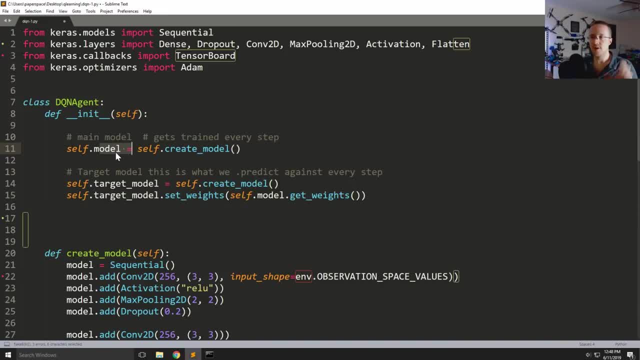 so this just keeps a little bit of sanity in your predictions, right? so in the predictions that you're making, this is how you'll have a little bit of stability and consistency so your model can can actually learn something, because it's just going to be. there's so much randomness. 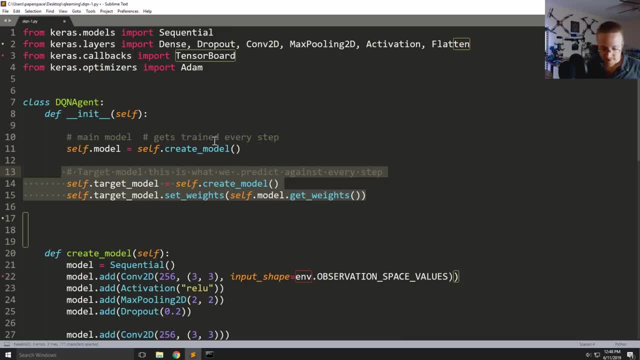 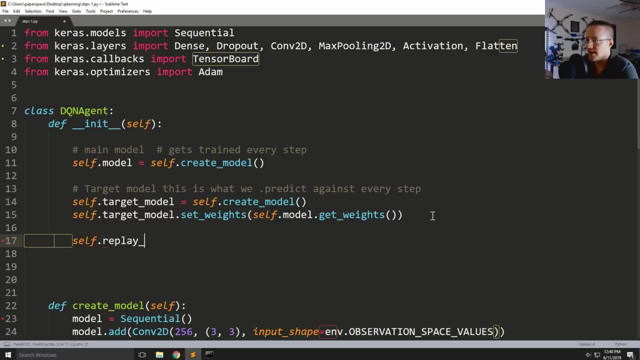 it's going to be very challenging initially and so long as you're doing things randomly, okay. so that's one way we are handling for the chaos that is about to ensue. next, we're going to have selfreplay, underscore memory and that is going to be a deque or deque. 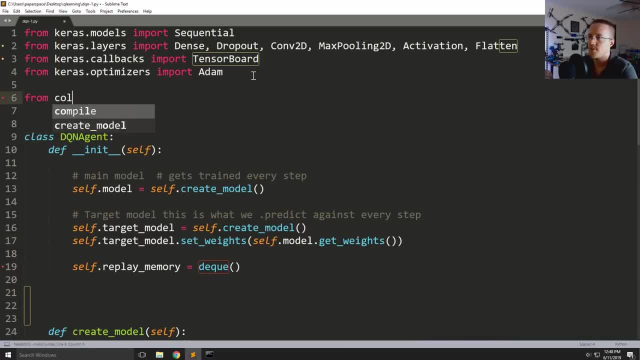 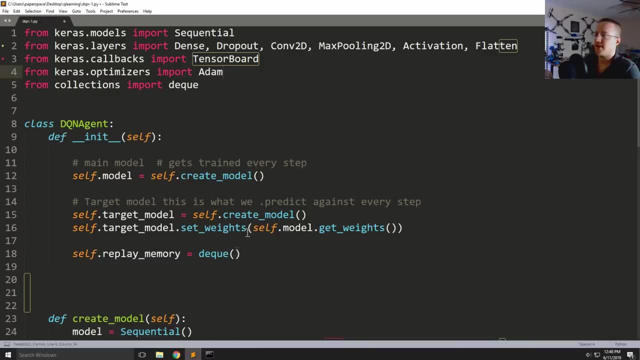 i don't. i always forget how to pronounce that um to use that we're going to say from collection, collections, import deque um, and if you don't know what deque is, it is a set length. think of it as like an array or a list that you can say: i want this. 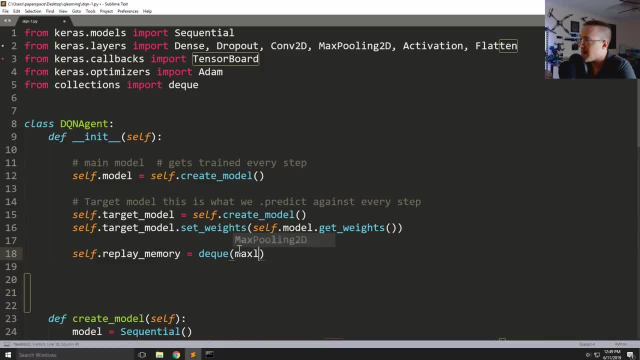 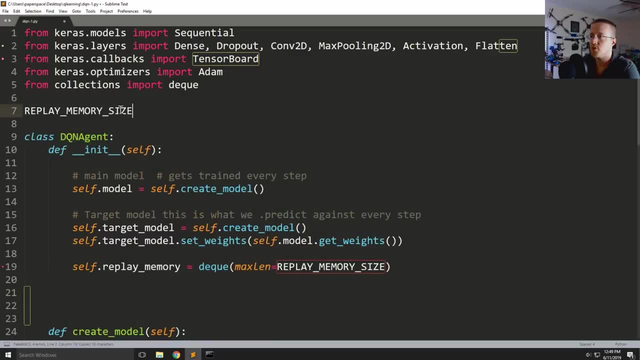 list to be a max size. so we're going to say max len equals replay memory size and let's go ahead and just set that real quick. we'll just say boom and we'll set this to um 50 000.. also a cool little trick i recently learned was you can use underscores in place of commas. so so, python c. 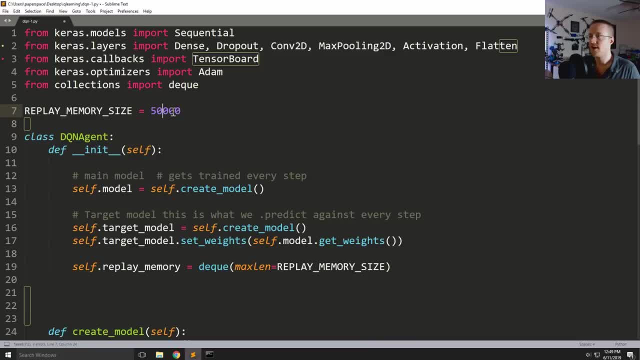 says 50 000, but it's a little more human. readable like this number is a little harder, but then, especially like once you have like a number like this, the underscore suddenly becomes very useful. so cool, so don't do a plus though. underscore. cool, so that's our replay memory size. so what? 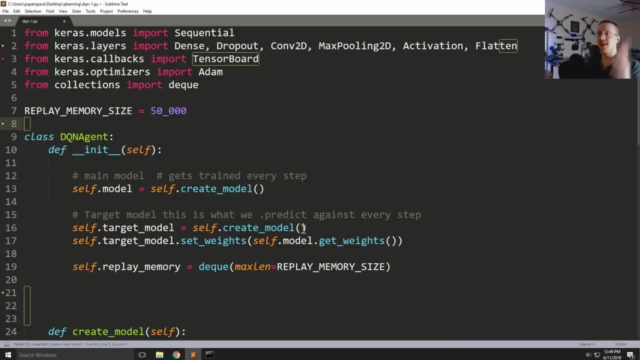 the heck is this? so the replay memory. so we talked about how we keep the predictions, so how we keep the agent taking consistent ish. so at least the agent is taking steps consistently. it's consistent with with the model over time. okay, i'm trying to think of a great way. 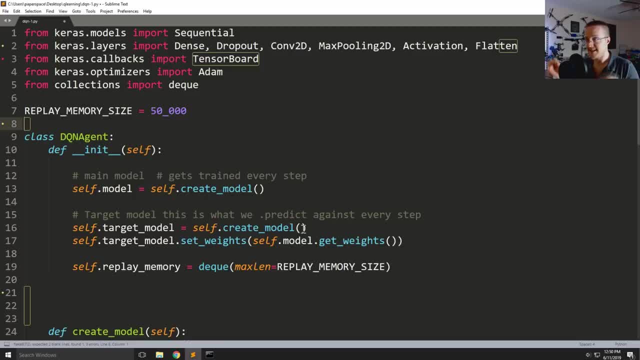 to word that. but so we've got the prediction consistently. consistency sort of under control. it's still gonna be crazy, it's at the start period. but this is that. we've got that settled. now we need to handle for the fitment craziness that is going to ensue because, because we so- 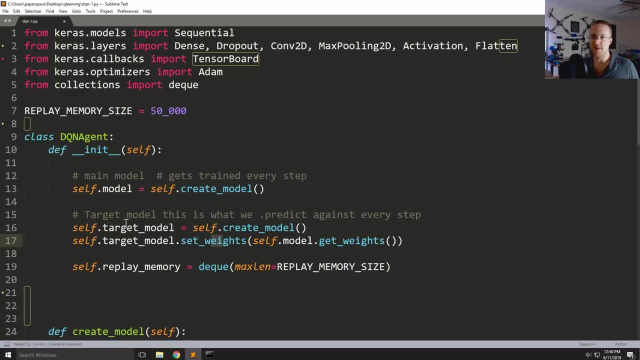 we have. you know, we've got two models so we've slowed down one, one way of working with that model, but the other one's still going to be crazy. so selfmodel still going to be dot fit every single step. But not only is it getting a dot fit every single. 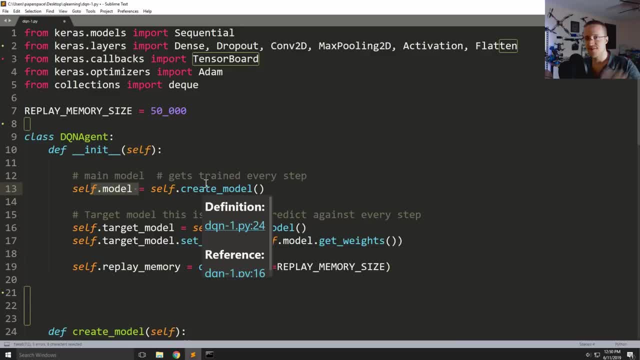 step. it's getting a dot fit of one value every single step. So again, assuming you're not new to neural networks, you know that we train neural networks with a batch, And part of the reason why we do that is one. it's quicker, but it also tends to have better results, not necessarily the higher. 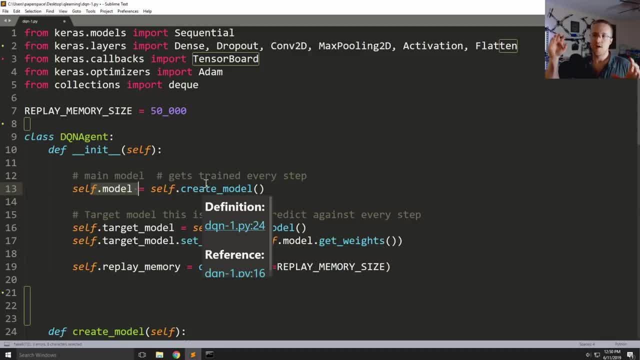 the batch you use. At some point the batch size gets too big. But to have some sort of batch size used, it generally will result in a more stable model and just learning over time. So if you just fit with one thing, it's going to adjust all those weights in accordance to that one thing. 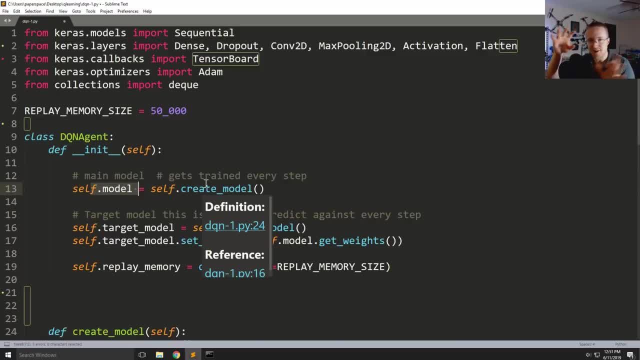 and then it's going to get to the new thing, do another fit, and it's going to adjust all the weights in accordance to that one thing, as opposed to if you throw in a batch of 64 things, it's going to adjust all the weights in accordance to all 64 things. 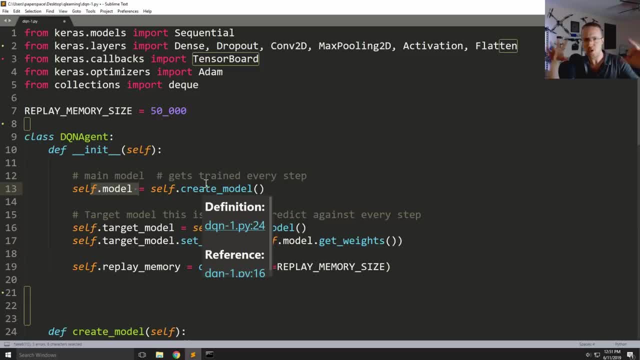 So it's not just the batch size, it's going to adjust the second batch And so the batch size not going to overfit to one sample and then go to the next sample and overfit to that sample and then go to another. you know what i'm saying? so, um, so we want to handle for that too, and the way that. 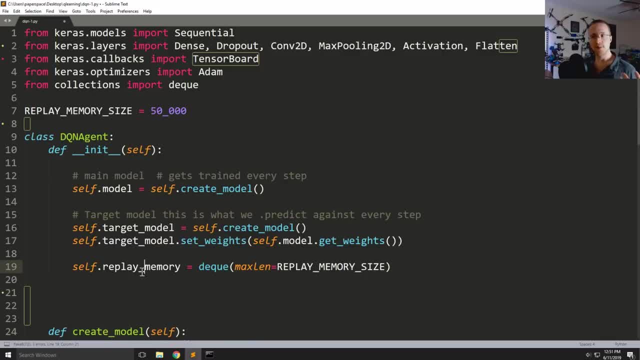 we do. that is, we have this replay memory. so we take this replay memory and that can be, let's say, 50 000 steps, okay, and then we take a random sampling of those 50 000 steps and that's the batch that we're going to feed off of, so train the neural network off of. so that's how we're. 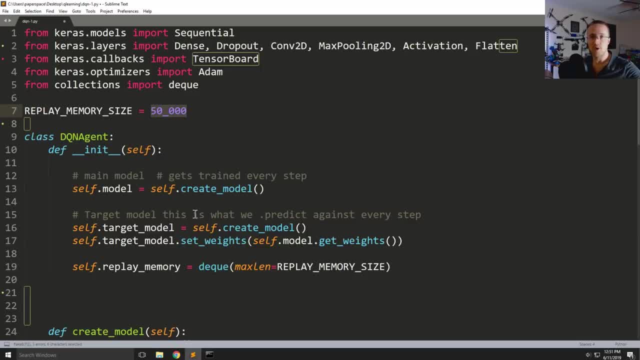 getting stability in both the training network that's getting updated every single step, but hopefully we're smoothing that out a little bit. and then we're smoothing out the predictions, because we're also not allowing the prediction model to be updated every step. instead it's being updated, let's say, every five episodes or whatever we intend to go with. these are all hyper parameters. 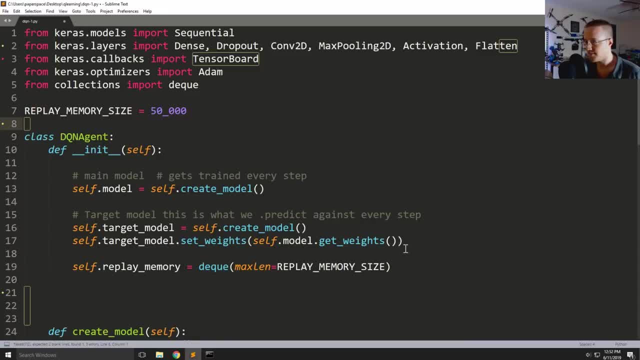 or really constants that we're going to set at the top of our program. okay, replay memory, okay. so the next thing is going to be selftensor, uh, tensor board, and that's going to be equal to modified tensor board, and we're going to set log, underscore, dir to be. 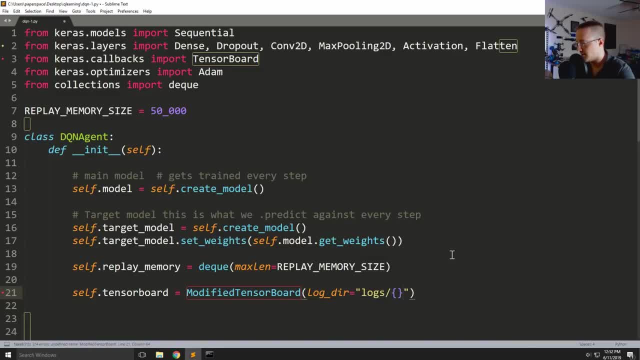 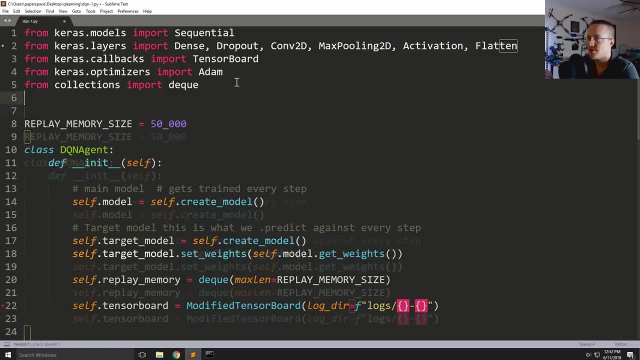 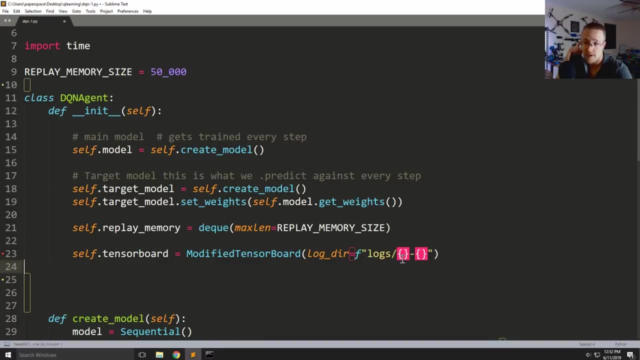 logs: slash uh var, dash var, and we're going to make this an f string and we're going to import import time. if you're uh want to say 3.5 or younger python, you can't do f strings, you'll have to do a dot format or whatever um, and so for the logs we're going to say model underscore name. 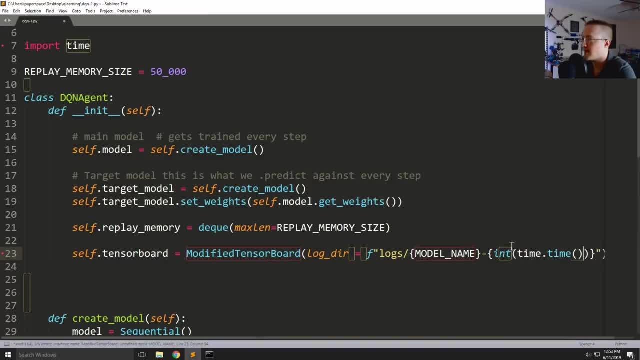 and then we're going to say: int time, dot time. this is just so we can kind of keep track of what's what. uh, and then the next thing i want to do- i thought it was getting pissy at me for this, anyway- uh, let's go ahead and set model name. 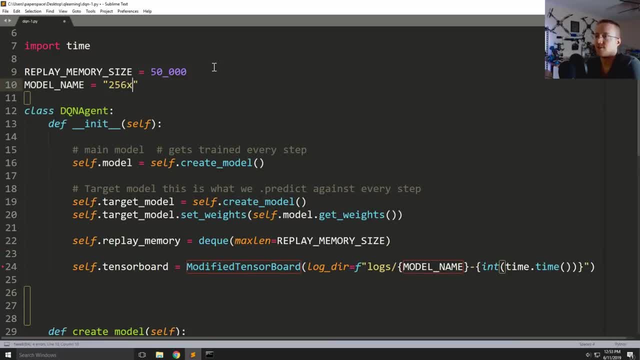 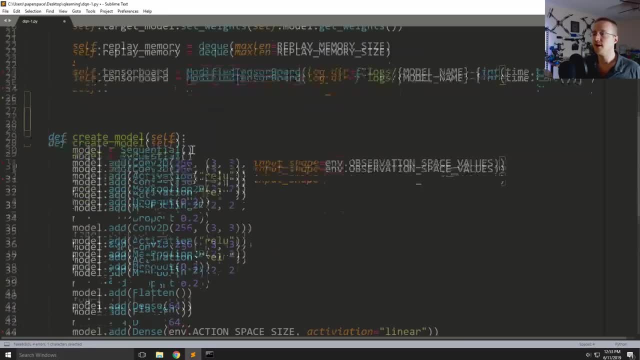 before i forget, and for now, just it's whatever you want. i'm going to say 256 by 2, because later you might try a 32 by 2 and a 64 by 2 anyways, and by 256 by 2 i mean the neural network. it's a 256. 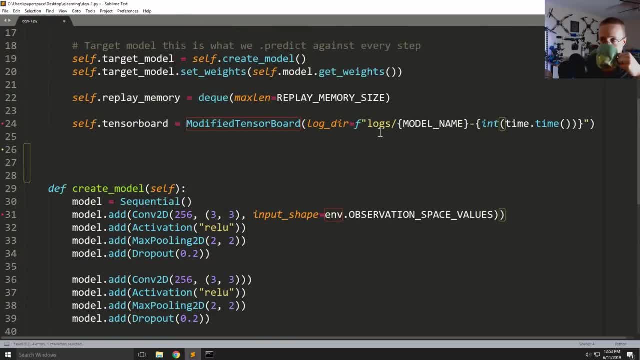 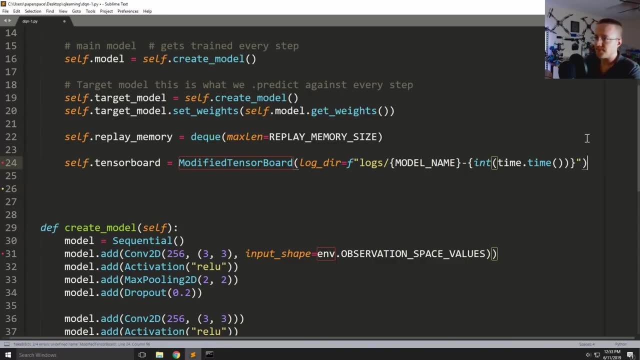 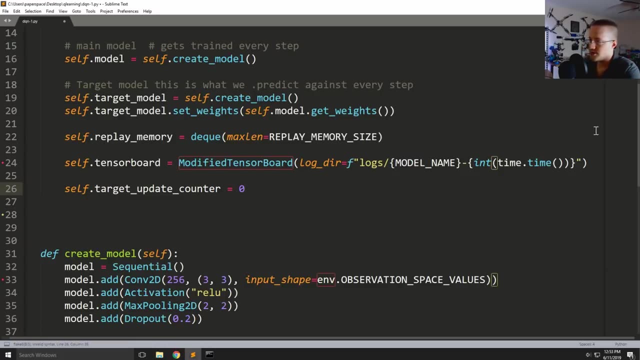 by 2 continent. so we've got um tensor board done. obviously, this doesn't yet exist. i'll talk about that in a moment. and then, finally, selftarget update counter equals zero, so we're going to use this to track internally um when we are ready to update that target model. 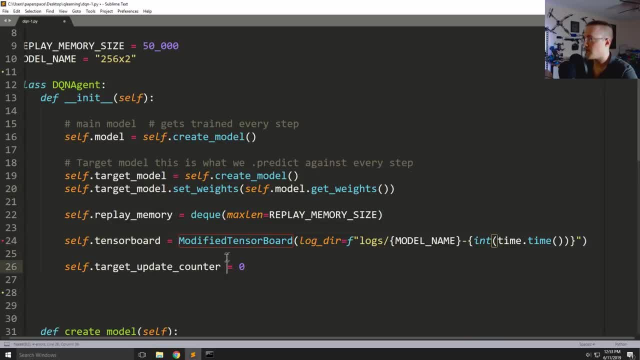 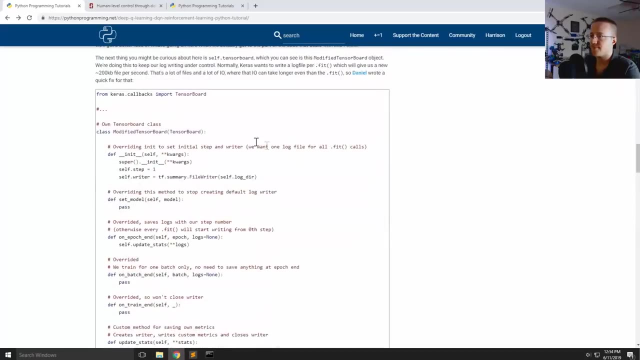 so this, you know this thing here, that we've explained why we want to do that. so, uh, the next thing we want is, um, i'm not going to write out that, so go to the text-based version of the tutorial and we're going to grab this updated um, this, uh, this updated tensor board class. uh, did we already? 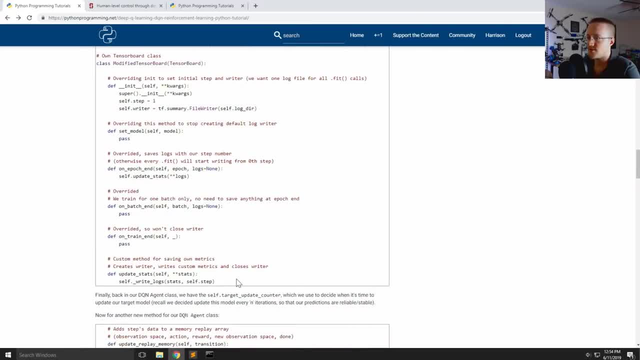 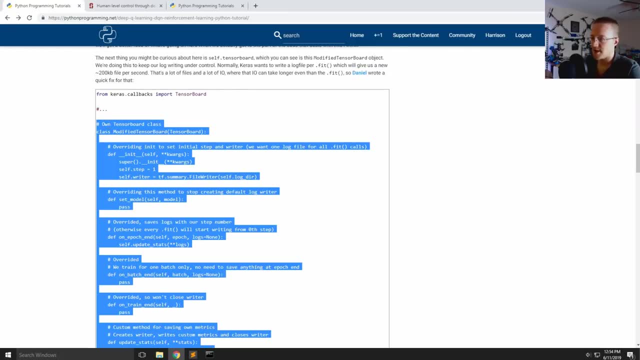 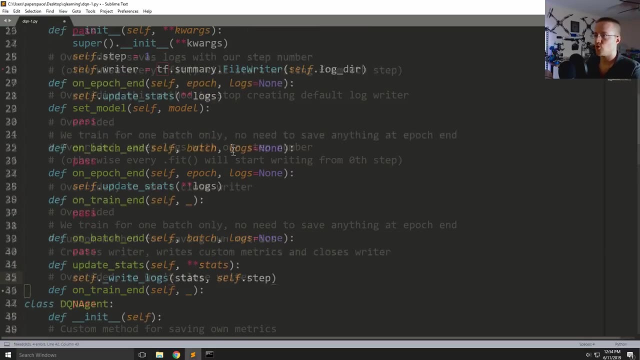 pull. i think we already pulled in tensor board. but what i really want is this right here: this whole uh class. i'm gonna- oops, i want that comment too. i'm gonna copy that. i don't really see any benefit for us writing that, but i'll explain why we want that here in a moment. paste that in, cool. so what this is doing is it's. 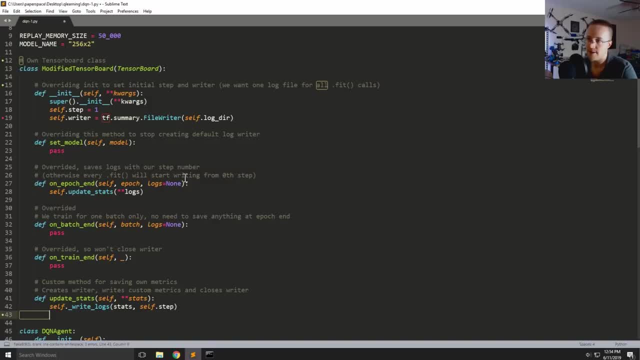 just modifying, uh, the tensor board functionality from tensorflow and keras, so by default, keras wants to update this, this tensor board file, this log file. every time we do a dot fit, well, we're doing a dot fit, uh, you know up, you know, about 200 times an episode, um, and then we're going to do like 25,000. 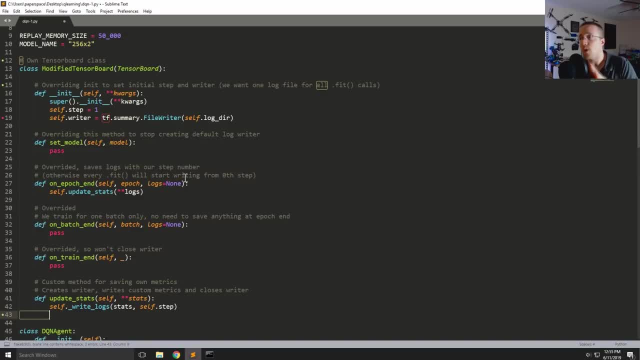 episodes. so first of all, i'm sorry, i think i used the word update log file. it wants to create a new log file per dot fit. well, we don't want that, we want just one log file. so, um so, having this is, as you can probably figure out, our inbuilt node. it will tell us: okay, i have a node, and then we've 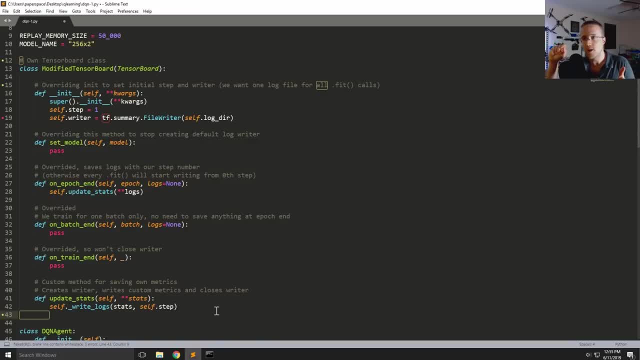 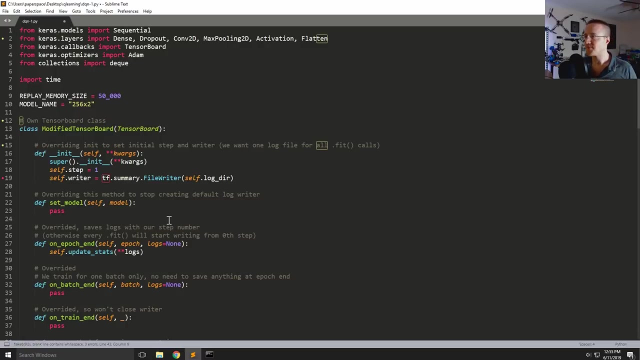 got status i'm going to gaming write d parce Berkeley. but then we can actually change that into in theometown. but basically in in счит we can't do that. it'll write a new node, arbnb big deal. but for deep q learning, where you're fitting just constantly um is something needed. 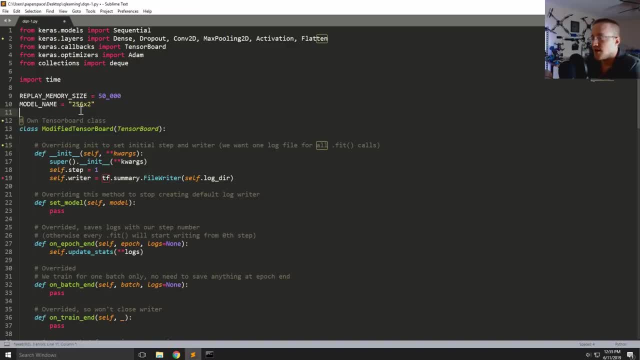 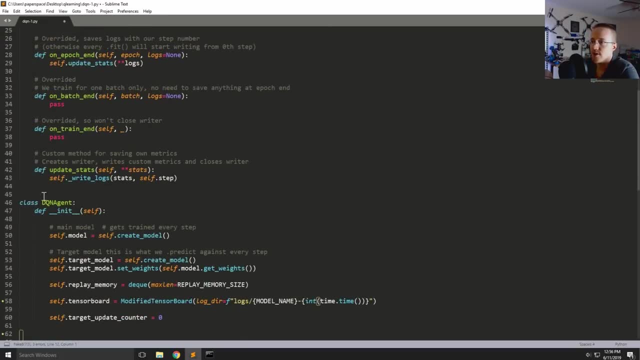 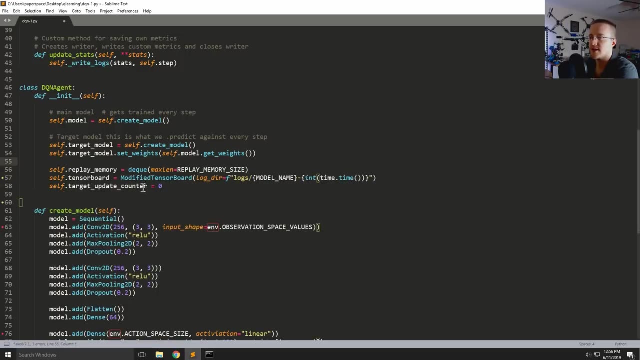 to be done. okay, so that is our modified tensor board. uh, now what we're going to do is go back to our dqn agent. um, so that's our init method. let me just kind of clean this up a little bit. i want these kind of separated out. uh, i don't want that separated out, i don't know. 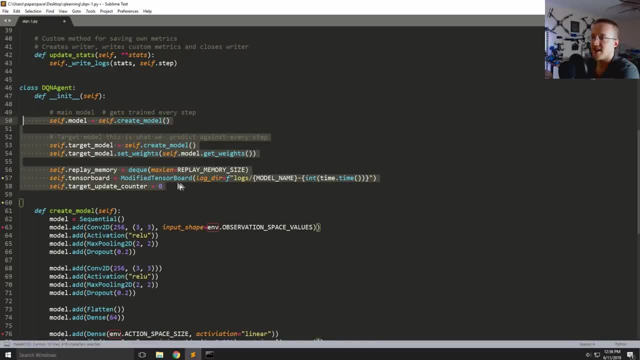 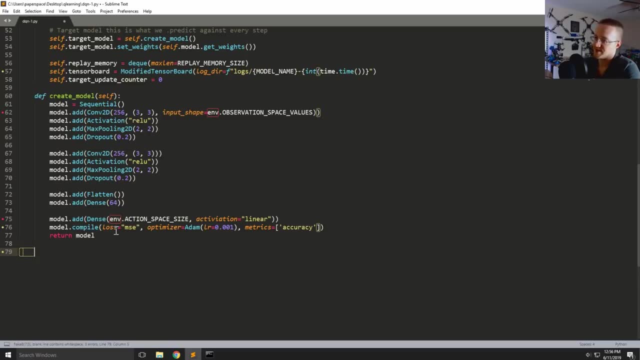 yeah, i can't really decide what i want, so i'll just leave that. so then create model. let's go ahead. let me see if i can, hopefully. well, we're not going to finish this, but let's add in one more method. so we're going to say define um, and in this one we're going to say: update underscore. 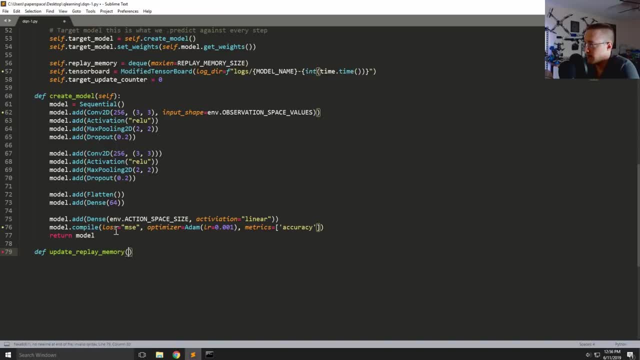 replay, underscore memory, uh, self, and then transition, transition, transition. can we type um? so then we're going to say self dot replay, underscore memory, dot append tran. wow, i really want to call that transition transition. so transition is observation is just going to be your observation space action, reward new observation space, and then whether or not it. 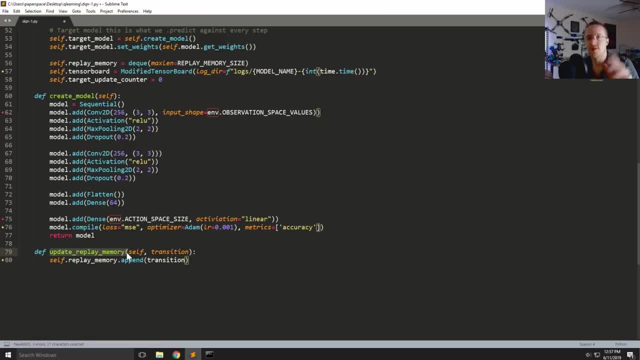 was done. so we need to do that, so we can do that new q formula. so that's that's all we're doing there. um, you'll, hopefully that'll probably make more sense when we actually get to actually use self dot update replay memory or agent dot update replay memory. uh, finally, um, yeah, we'll do, we'll do. 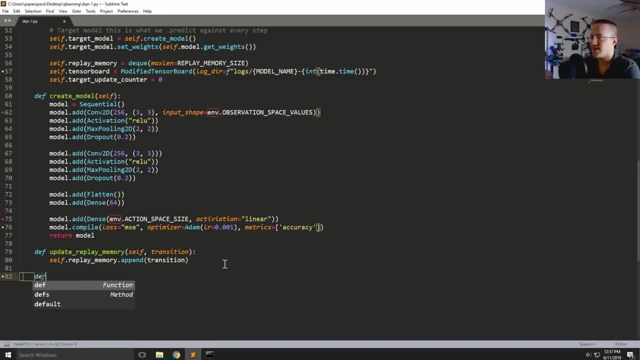 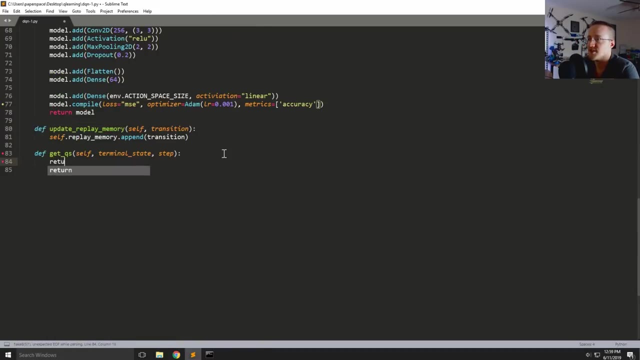 this one last method and then we'll save train for the next next tutorial. so that's going to take a while. so define: uh, get queues, so we will get queues, self terminal, terminal state and then step and then so this will be: return a whoops, self dot model underscore, uh predict, and we're going to say the. 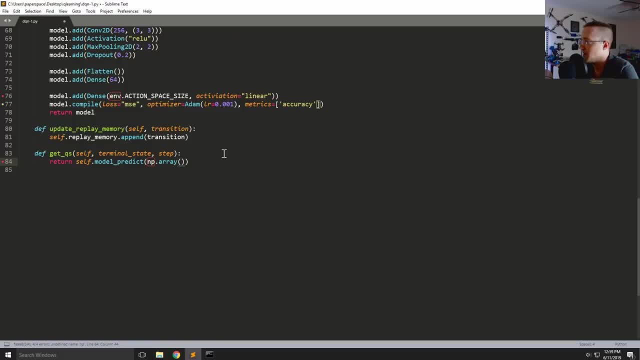 numpy array. i don't think we've imported numpy. we'll grab that soon. um of the state dot reshape, uh, negative one, and then we're gonna say asterisk state dot shape. all that's doing is unpacking state um. and oh did i? i sure did. terminal state, that's for train. right now we're just passing state here. 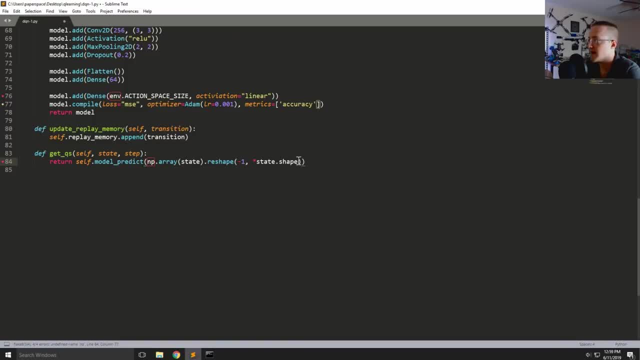 so state dot, shape and um, and then we're going to do div, whoops, div by 255, predict and then zero. so model dot predict always returns a list. even though in this case we're really only predicting against one element, it's still going to be a list of one element or an array. 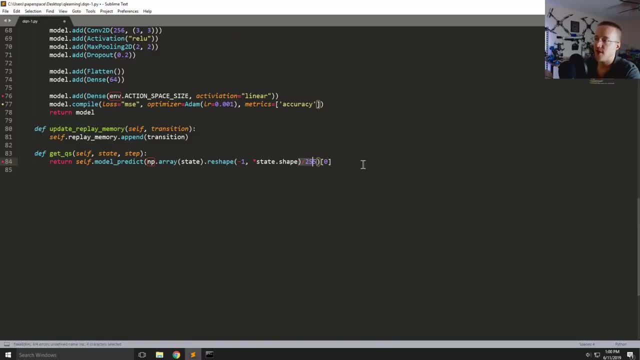 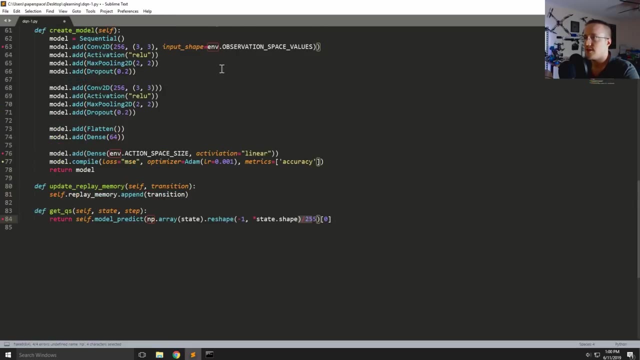 so we still want the zeroth element there. div by 255 is because we're passing in this rgb image data, so you can very easily normalize that data by just simply dividing by 255.. okay, so that's it. let's go ahead and go up to the very top here. let me import numpy as np. 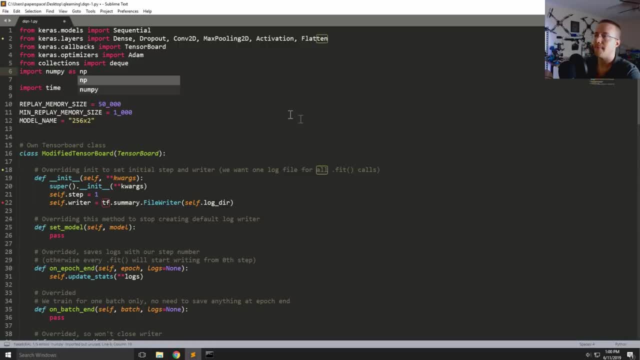 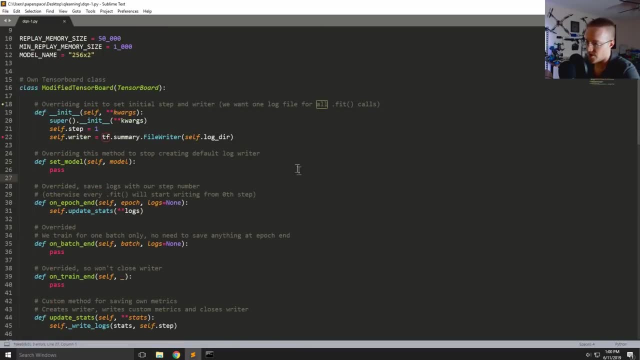 so let's say import numpy as np. let me go ahead and save that and i think i'm going to save train for the next tutorial, because that's going to take a while. So quick shout out to the recent- well, not recent actually. 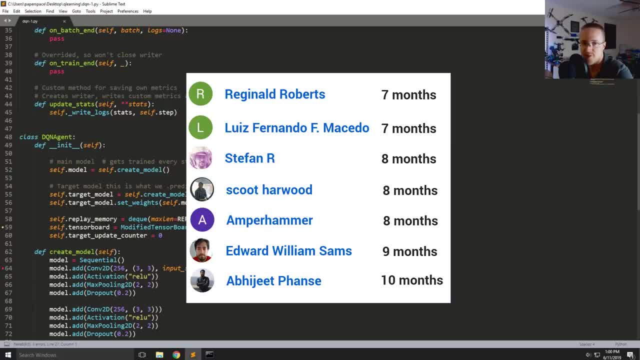 These are my long-term channel members, people who have been sticking around for a while: Reginald Roberts, seven months. Luis Fernando, seven months. Stephan R Scoot Harwood, eight months. Amper Hammer, eight months. Edward William Sams, nine months. 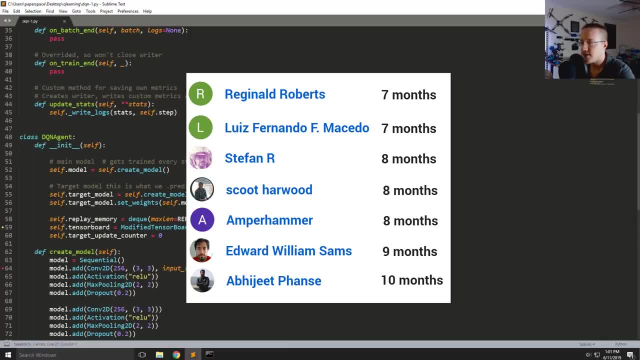 And Abhijit 10 months. That's quite a while, you guys. Thank you guys all for your support. Um, and if you guys have any questions, comments, concerns whatever, feel free to leave them below. If anything up to this point is confusing. 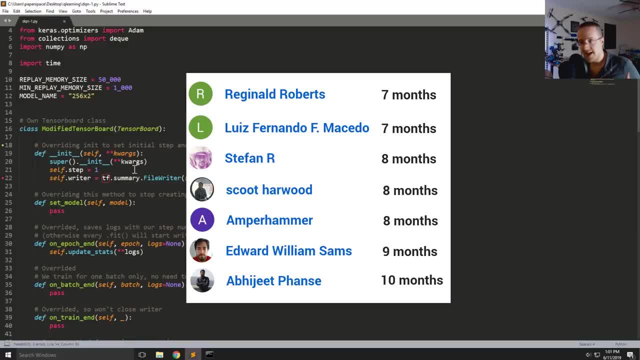 or you want to get a little more information again. comments below or come join us in discordgg. slash SendDucks. If you think I've done something wrong or said something wrong- I'm sure I have- Feel free to let me know. 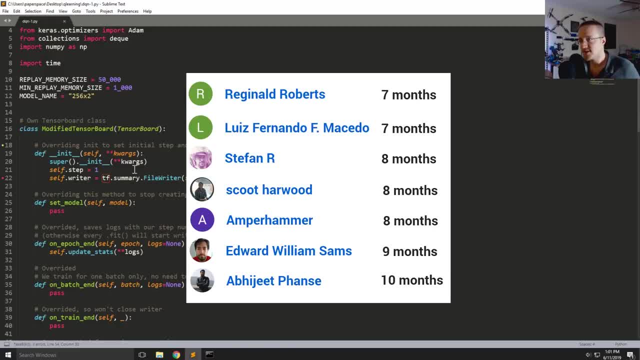 And, yeah, I'm hoping that you guys can get through this tutorial. seriously, I think right now I, just like I said, I could not find a tutorial or any information to actually do this kind of stuff that actually made sense or actually explained everything. 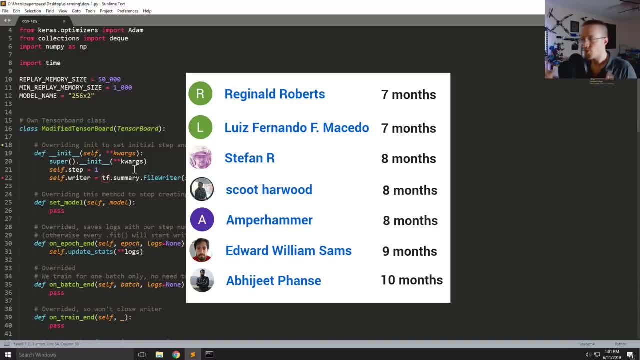 So just a lot of copying and pasting going on. So my hope is that you guys can actually get through this and know how to do this yourself. So that's my goal. So if you're having trouble getting to that point, let me know, because I need to fix that. 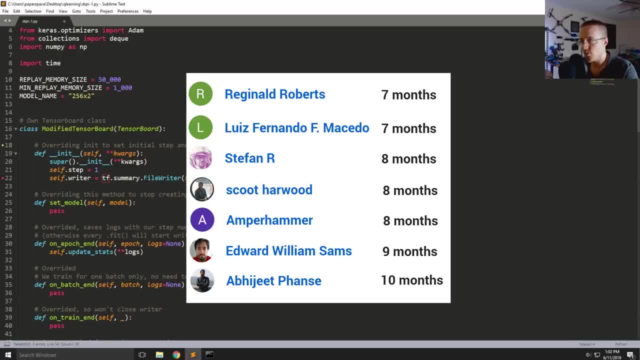 So, anyways, I will see you guys in the next video Where we will do the train method, and then we might only do the train method, but hopefully we can do the environment. I'm thinking I might just copy the environment. We made some tweaks to the environment.